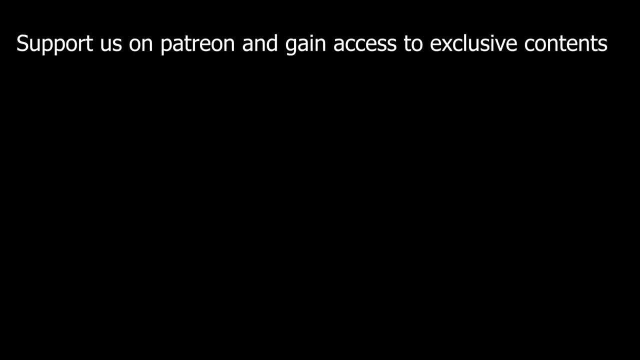 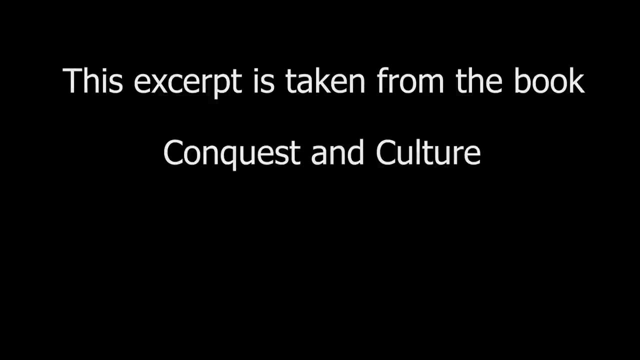 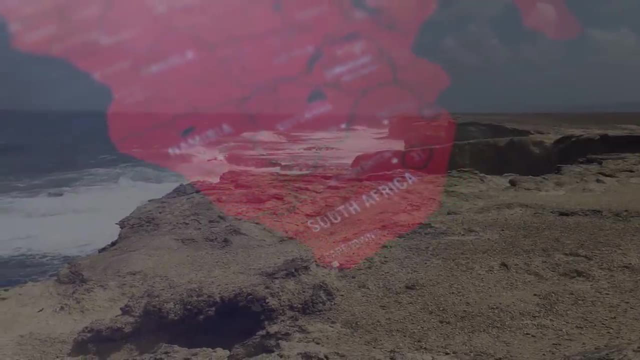 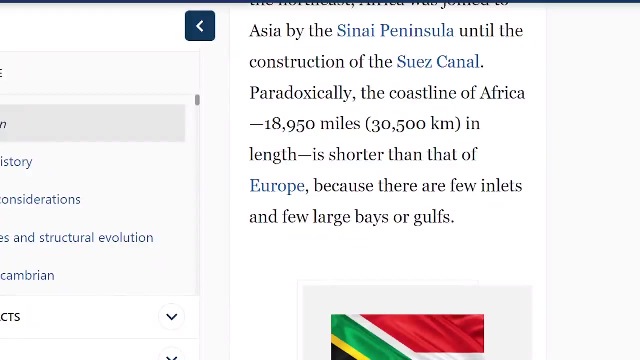 Thank you for watching. Africa is second only to Asia in size. This anomaly reflects Africa's lack of the numerous coastal indentations which form natural harbors in Europe, providing places where ships can dock, sheltered from the rough waters of the open seas, thereby enabling European countries to 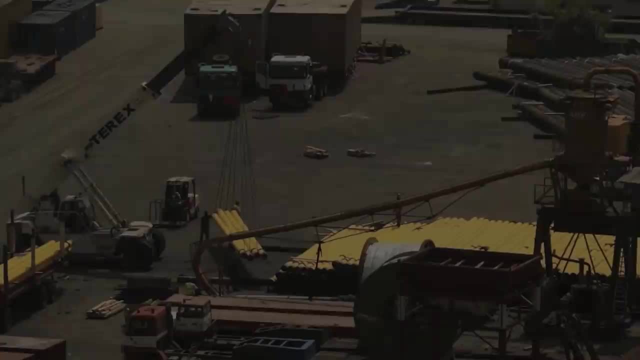 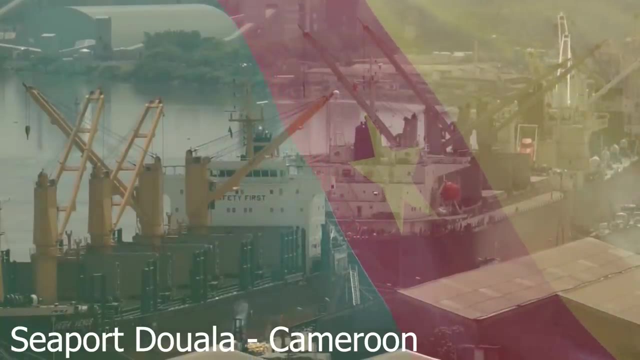 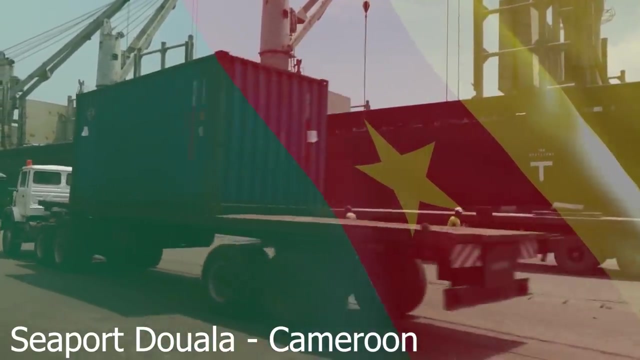 become maritime nations early in their history. In addition to a dearth of harbors, parts of sub-Saharan Africa have shallow coastal waters, so that maritime trade has often had to be conducted by the costly method of having ships anchor offshore with their cargoes being unloaded. 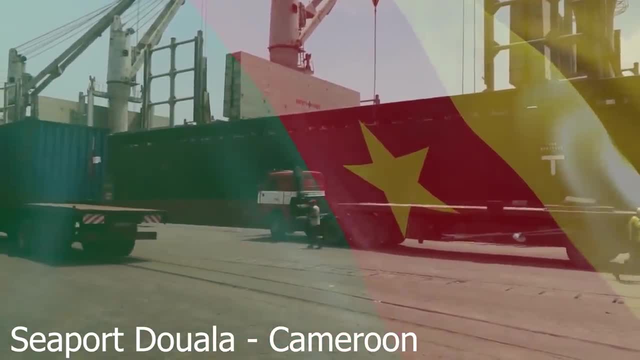 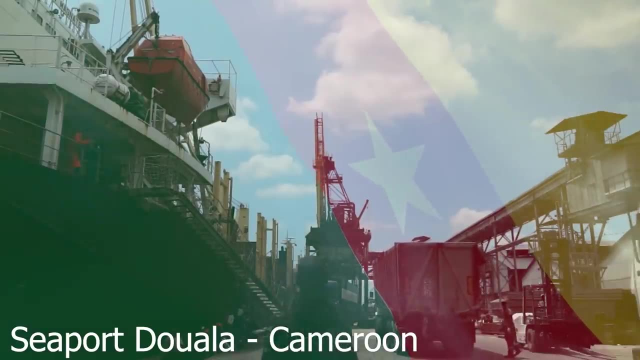 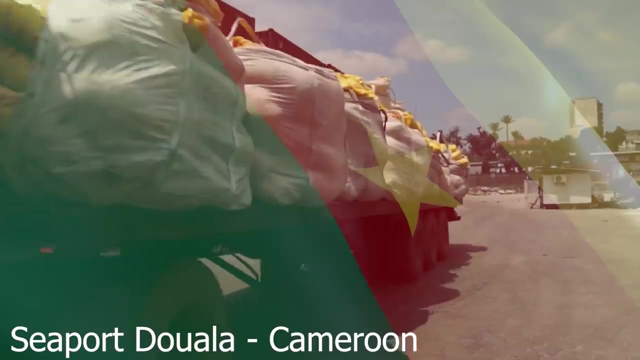 onto smaller vessels, which could then make their way to land through these shallow waters. Africans have generally not been seafaring peoples, except in the Mediterranean or in parts of East Africa, where these geographic constraints have not been as severe. Much of Africa, and especially sub-Saharan Africa, has developed without the benefits. 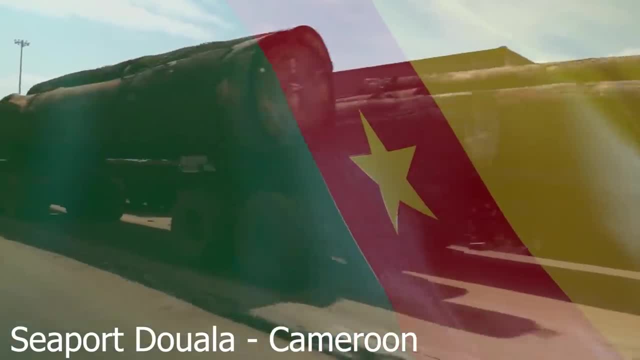 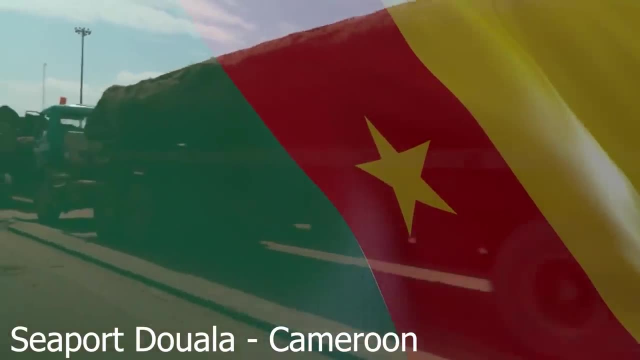 of a large maritime trade and the consequent stimulus of economic and cultural interchanges on a large scale with various and disparate peoples. While there has been for centuries some trade between sub-Saharan Africa and Europe, or with the peoples of North Africa and the 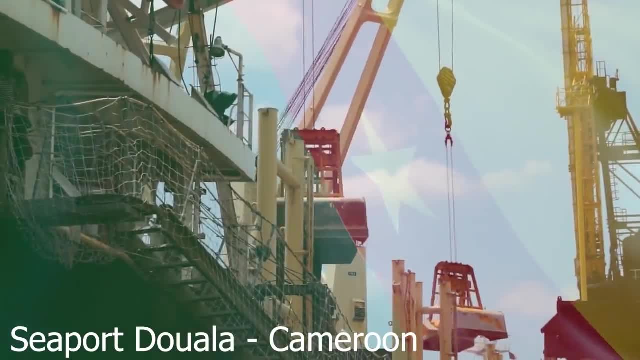 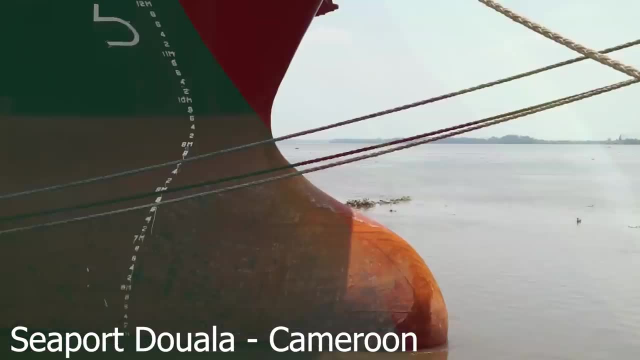 Middle East international trade has generally played a relatively smaller part in the total trade of Africa as compared to other continents, not only because of a dearth of harbors, but also because of a dearth of navigable rivers reaching into the interior of the continent from the sea. 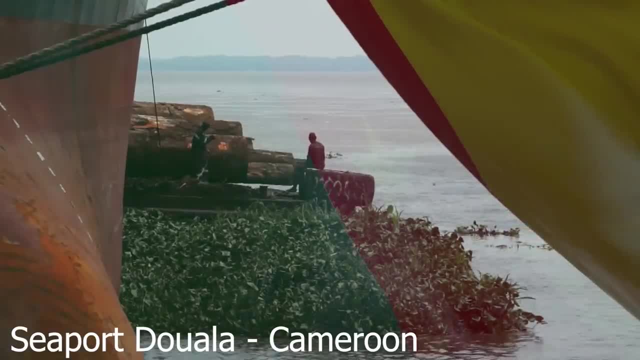 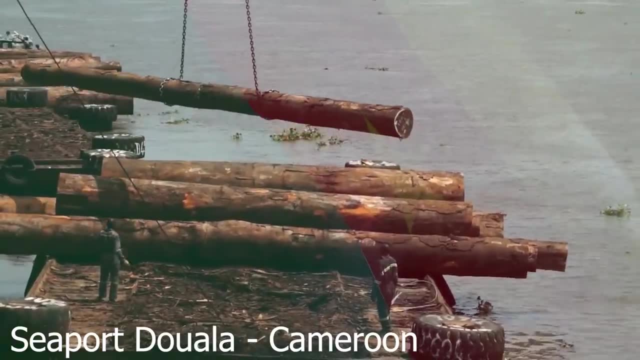 River mouths opening into the sea have been blocked by sandbars in some places, and in other places the few good harbors have been connected to hinterlands that were not very productive and so have had little to offer in trade. Thin coastal plains. 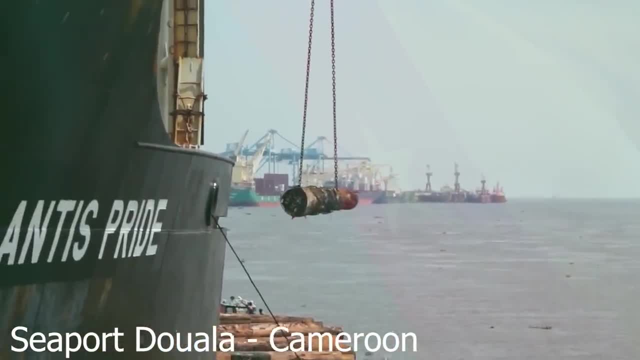 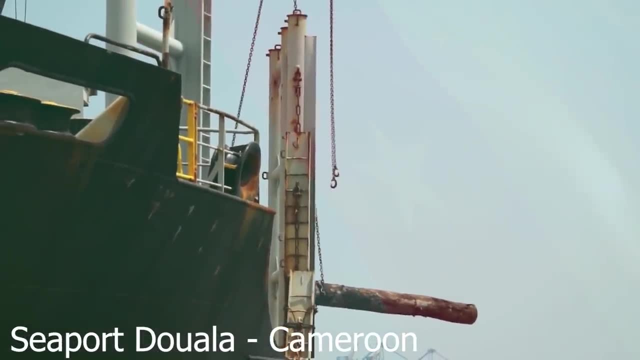 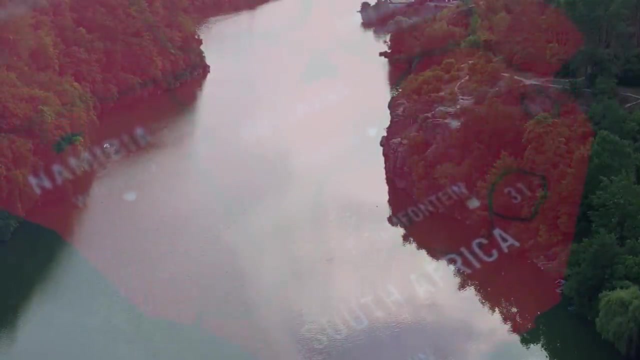 averaging only twenty miles in width and often backed by steep escarpments, have likewise provided little basis for large-scale international trade, even where other conditions might permit it. Low and irregular rainfall over many parts of Africa fill rivers and streams to a navigable. 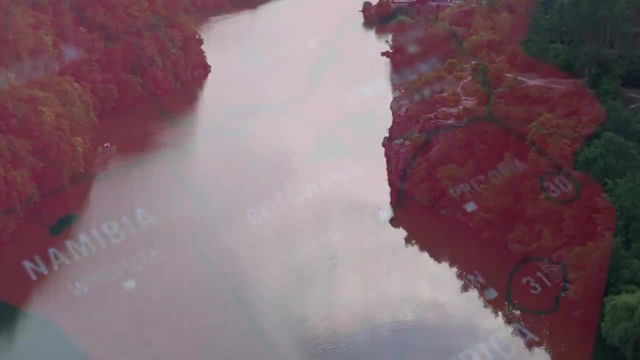 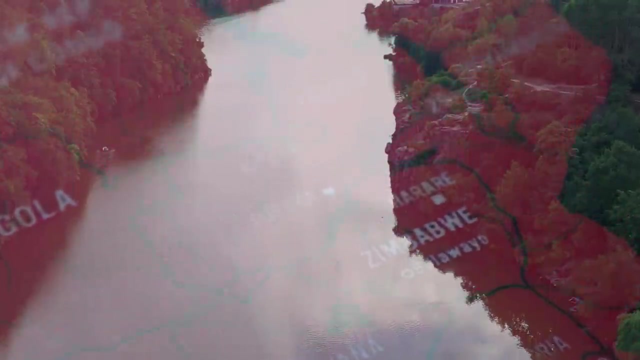 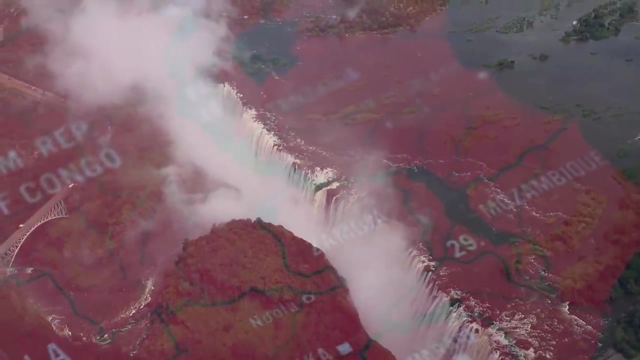 depth only intermittently, and even when filled. many rivers and streams are navigable only by smaller boats or barges, not ocean-going vessels. Where the volume of water is sufficient for navigation by sizable vessels, the many rapids and waterfalls of Africa still impede. 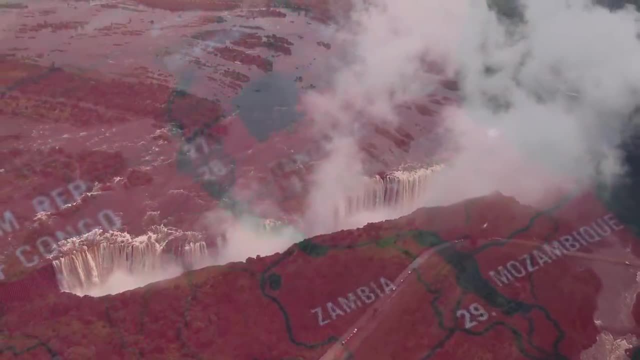 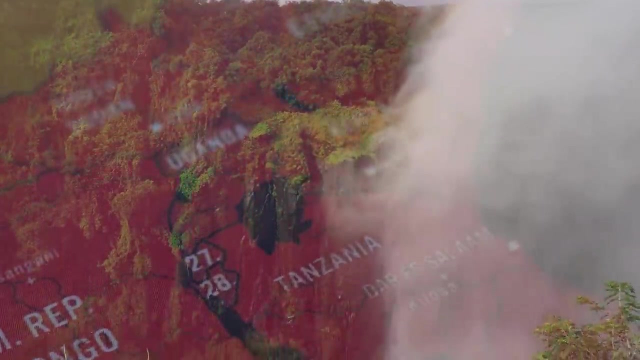 international trade. The Zaire River, for example, is twenty-nine hundred miles long and has a volume of water second only to that of the Amazon, but its rapids and waterfalls near the sea prevent ocean-going ships from reaching inland. Thus the role played by 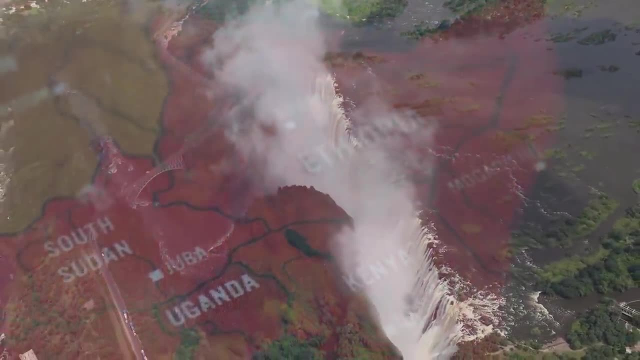 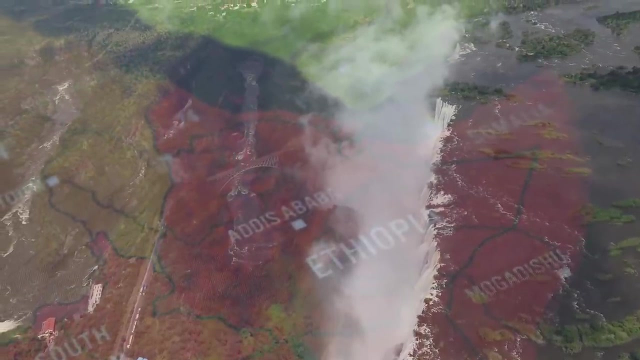 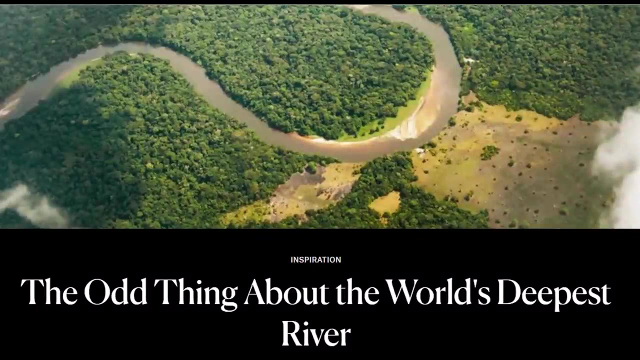 other great rivers of the world in facilitating the development of ports that became great cities, contributing to the economic and cultural development of the surrounding lands and peoples, was denied the Zaire by the intractable facts of geography. Nor is the Zaire unique among Africa's rivers. 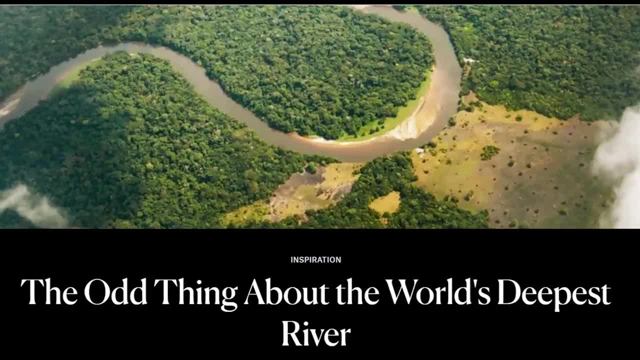 Nor is it unique among Africa's rivers. No river in sub-Saharan Africa reaches from the open sea to deep into the interior. On the Mediterranean coast, only the Nile reaches far inland Significantly. the Nile spawned the most famous of the civilizations developed on the African continent, as well as the two 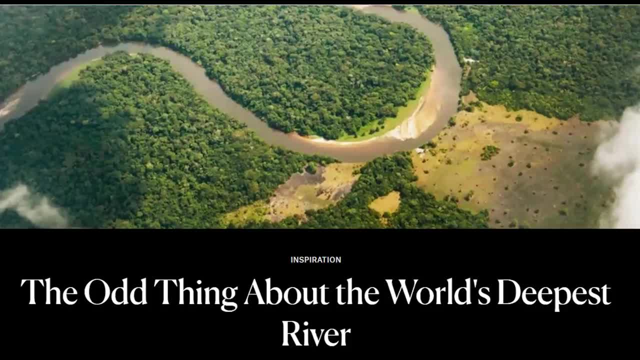 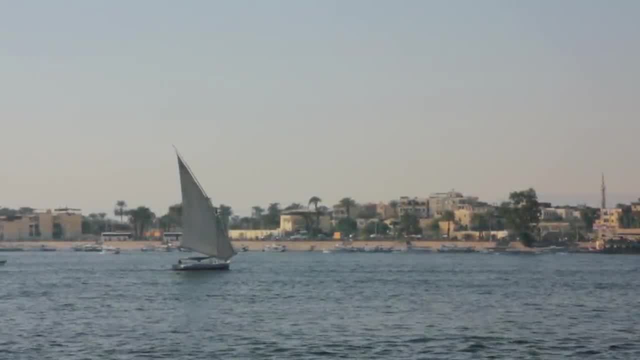 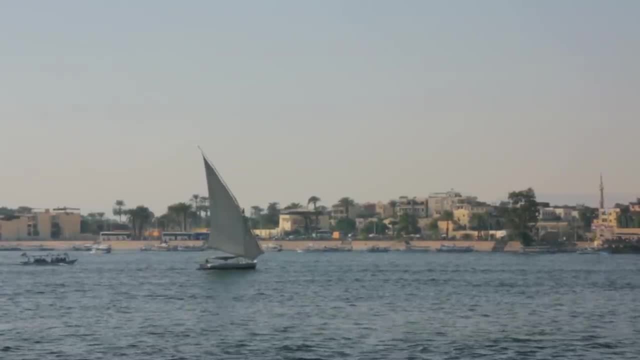 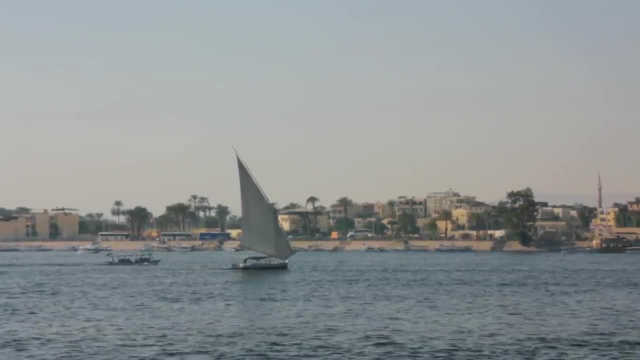 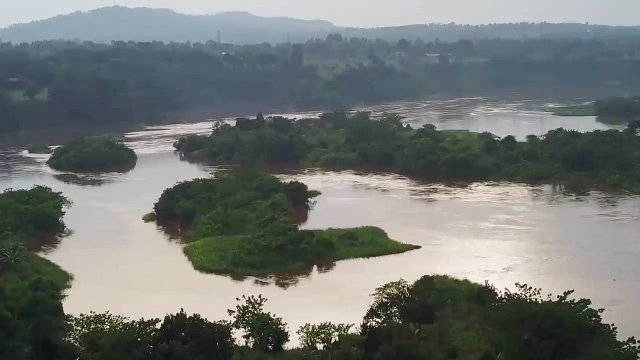 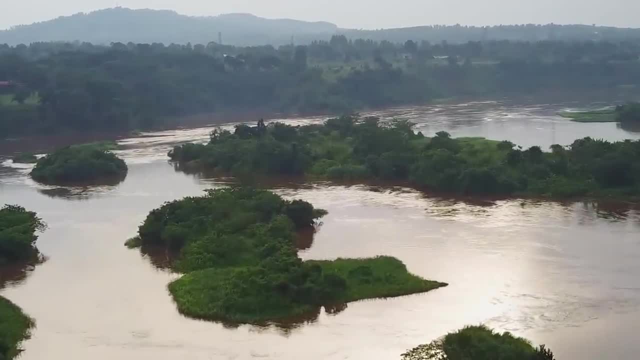 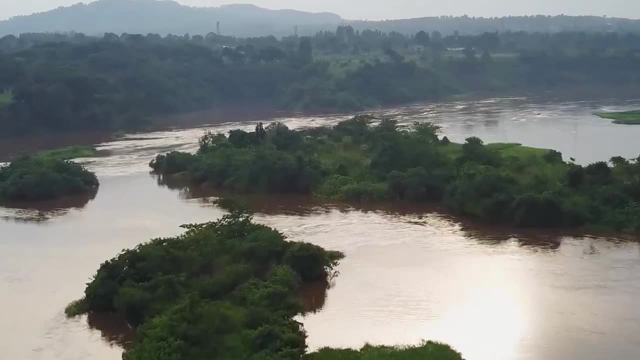 fewer of them in Africa, which has been and remains the world's least urbanized continent. Among the relatively few things which have had sufficiently concentrated value in a relatively small physical size, the Nile, which has been and remains the world's least urbanized continent. 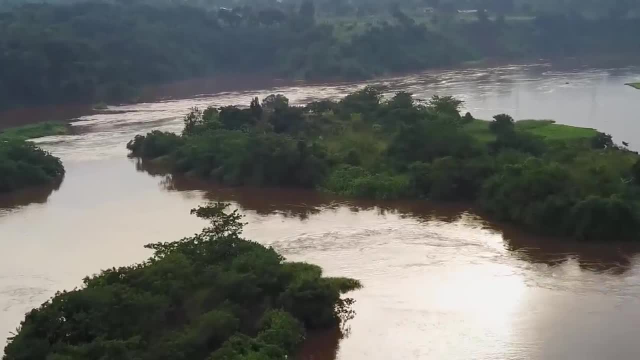 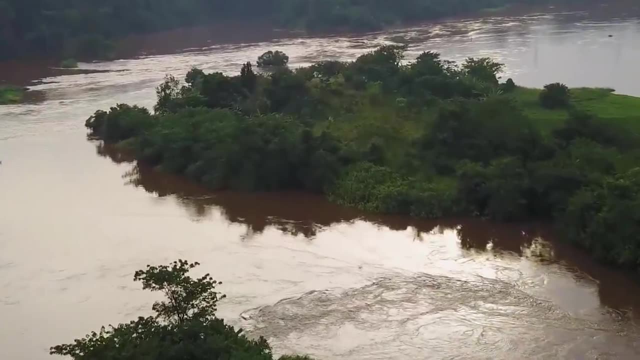 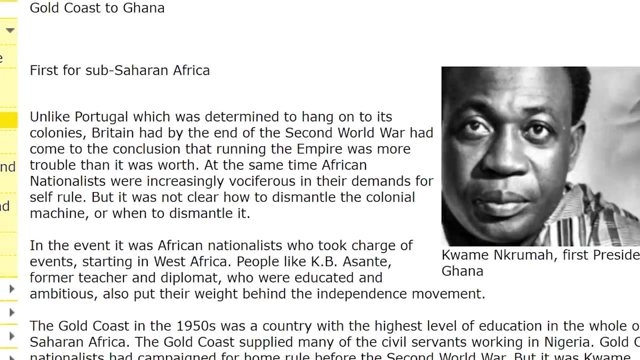 so as to be able to repay the high costs of transport from Africa have historically been gold, ivory and slaves. All three became major exports. The coast of what is now Nigeria became known as the Slave Coast, just as the coast of neighboring Ghana to the west was called the Gold. 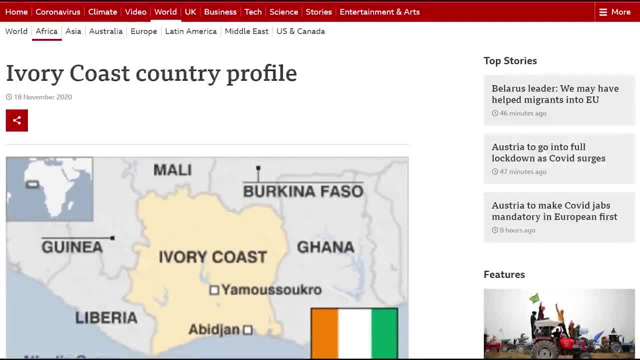 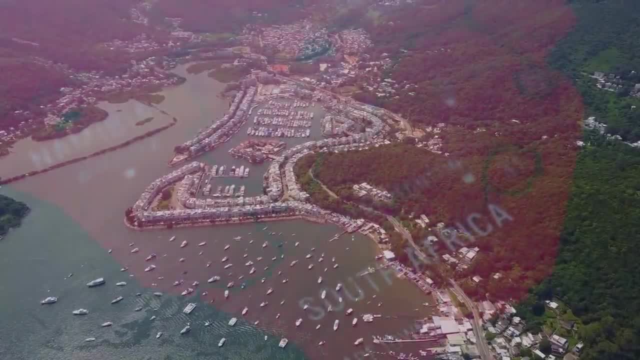 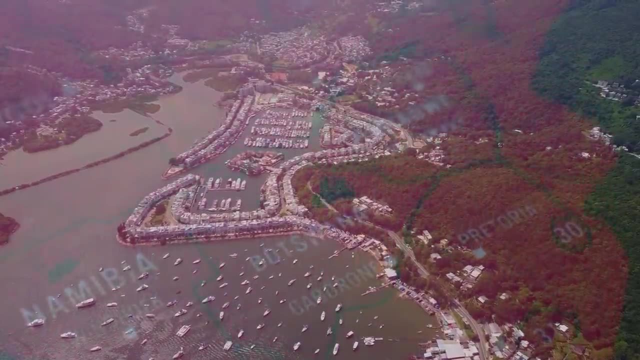 Coast and that west of Ghana was and still is called the Ivory Coast. One indicator of differences in access to waterways is that, while more than a third of Europe's landmass consists of islands and peninsulas, only two percent of Africa's landmass consists of islands and peninsulas. 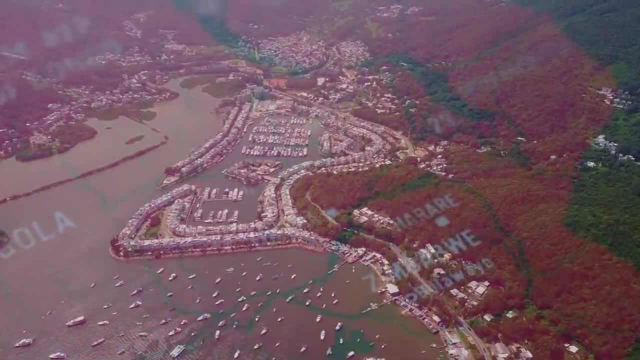 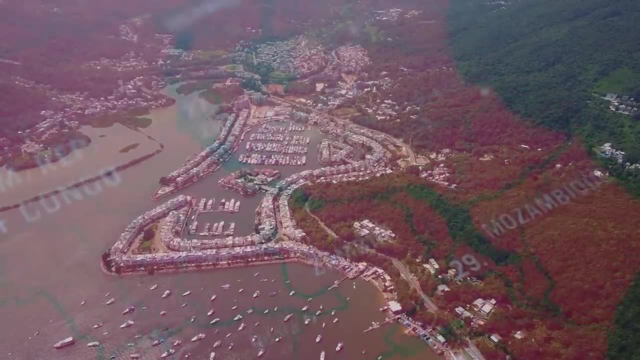 Such disparities in access to waterways are accentuated when the navigability of these waterways is also taken into account. Even the Niger River, the heart of a great river system in West Africa draining an area nearly twice the size of Texas, is not navigable everywhere by 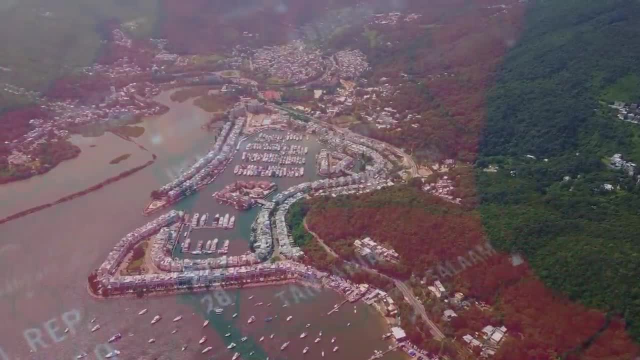 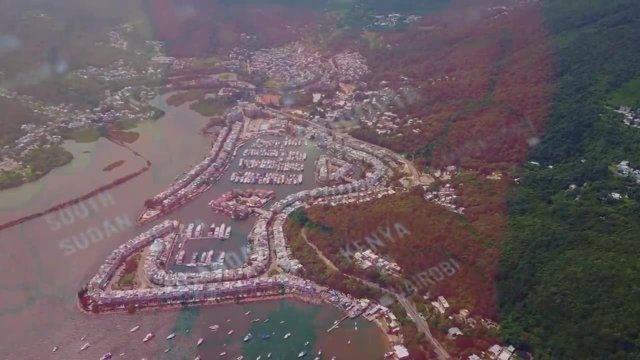 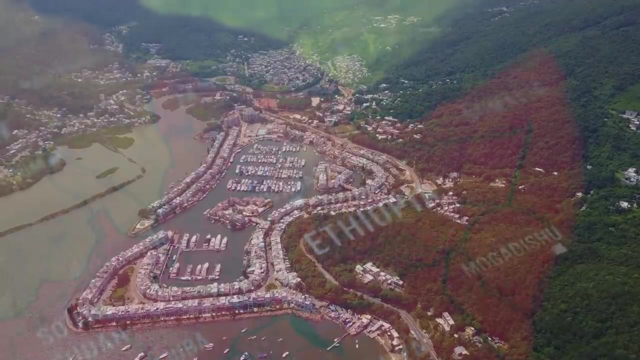 large rivers, vessels and is not navigable at all in some places because of rapids. At the height of the rainy season, the Niger may become a twenty-mile-wide moving lake, but during the dry season, the average depth of the Niger can, in places, fall below four meters. Despite its serious limitations, 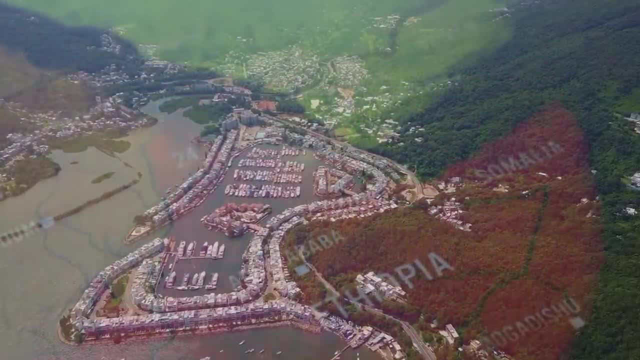 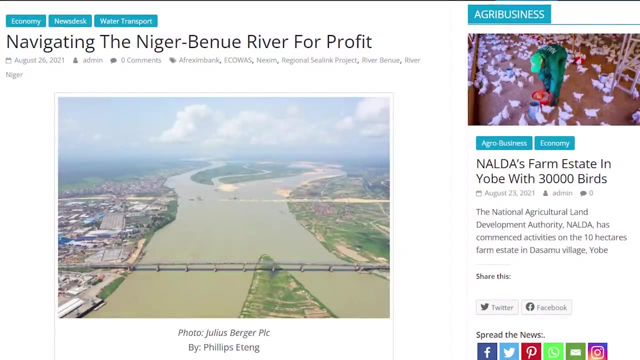 the Niger compares favorably with other African rivers, with even more serious limitations. The Niger has been characterized as the easiest to navigate in all of tropical Africa. navigating the Niger's chief tributary, the Bainway River, for example, has been more. 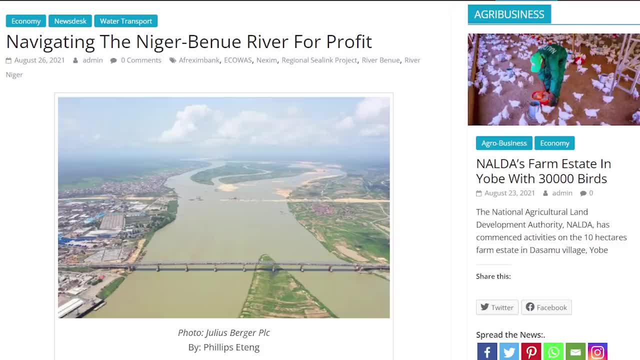 problematical Because of seasonal rainfall patterns. the upper Bainway has been navigable only two months of the year, leading to hectic and complicated shipping patterns. If they let the craft stay up the Bainway a day too long, the vessels will be stuck on sandbars for ten months. 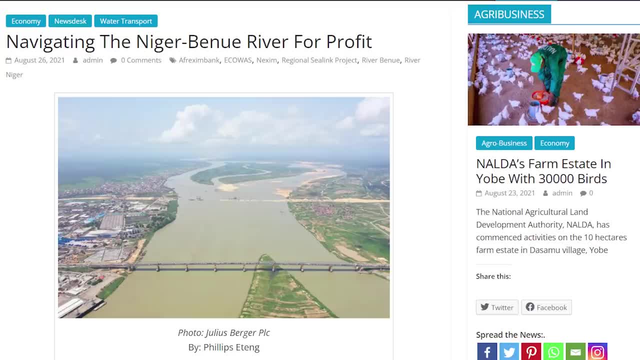 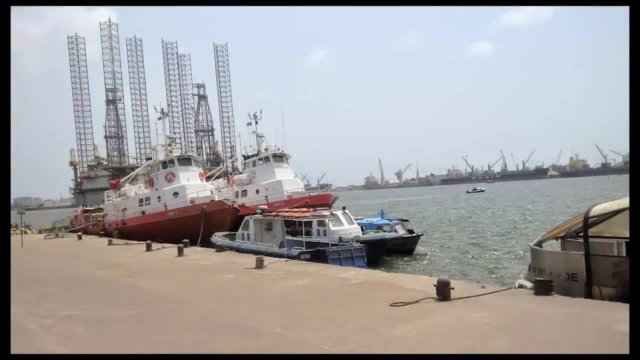 Yet if, through caution or misinformation, they withdraw the fleet too soon, much valuable merchandise is left behind. The Niger can only be evacuated by land at much greater cost. The first boats to go in are the commercial canoes, then follow the larger craft and finally, when there is sufficient water, at 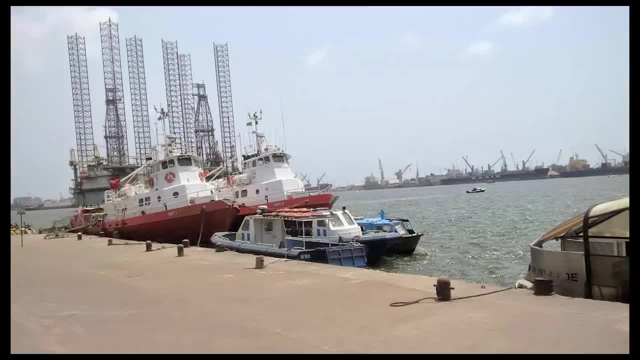 Locoja. the largest power craft and their barges sail up the river as fast as possible Towards the end of the short season. the large craft have to come out first because of the fall in the level of the water. The medium-sized craft follow and the small canoes may continue for some time. 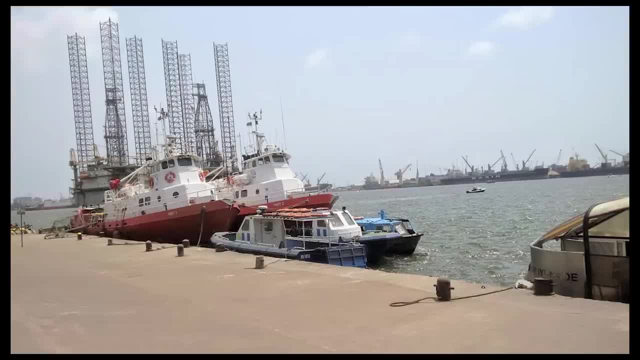 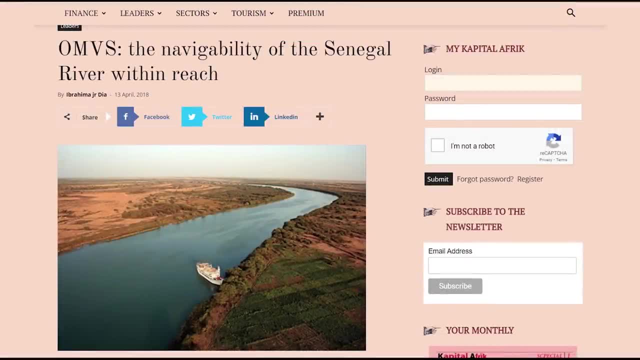 So they are prepared to avoid any major damage to an ancient ship and all the others. Drastic changes in water level are common in other West African rivers and streams. The Senegal River has been characterized as precariously navigable And only during some months. 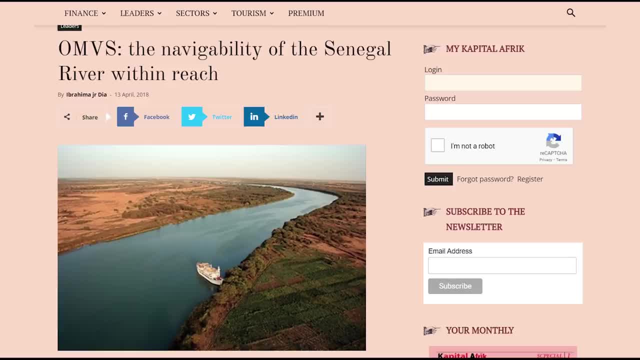 at that. Like the Niger, the Senegal is not only subject to large seasonal changes in water flow, but also contains rocks and rapids. In East Africa, such rivers as the Zambezi are navigable only five times in a day. 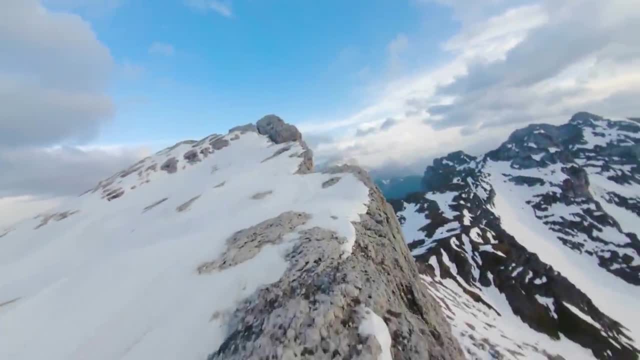 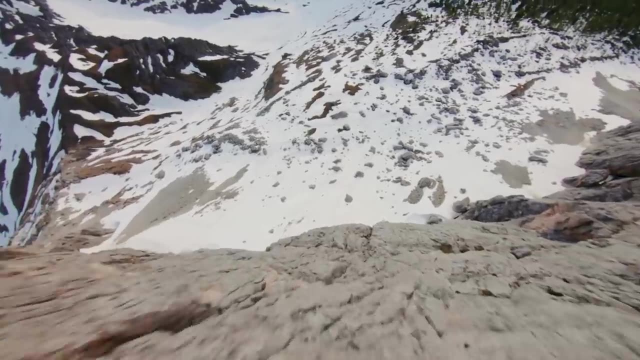 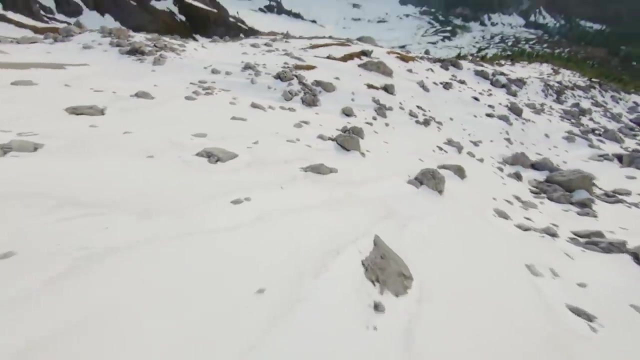 relatively short stretches. one reason for the drastic seasonal changes in water levels in african rivers is that tropical africa is one of the few large regions of the world without a single mountain range to collect snow, whose later melting would supplement rainfall in maintaining the flow of streams and rivers. rivers in tropical africa are wholly dependent on rainfall, and that 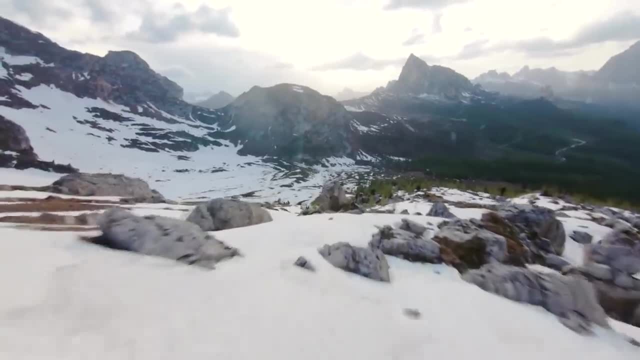 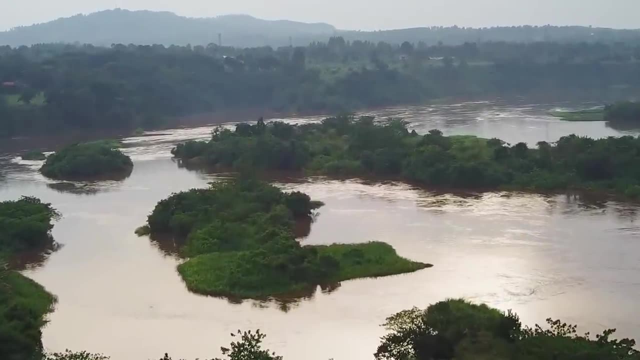 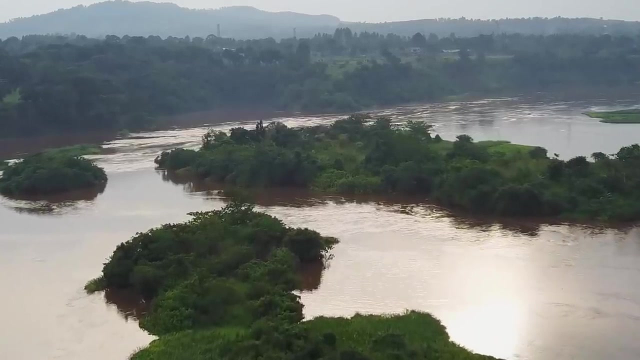 rainfall is itself highly undependable, not only from one season to another, but also from one year to the next. the term navigable can, of course, mean many things. in some of the rivers of angola, for example, it means navigable by boats requiring no more than eight feet of water and, in parts, 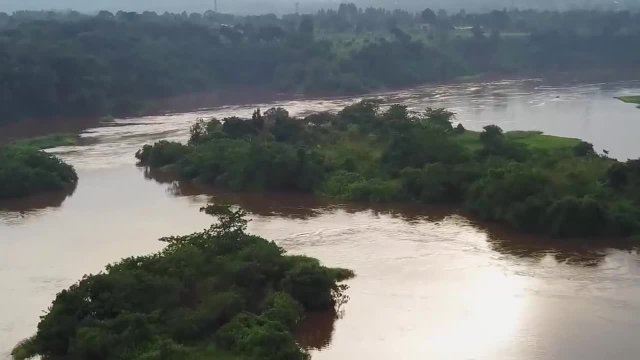 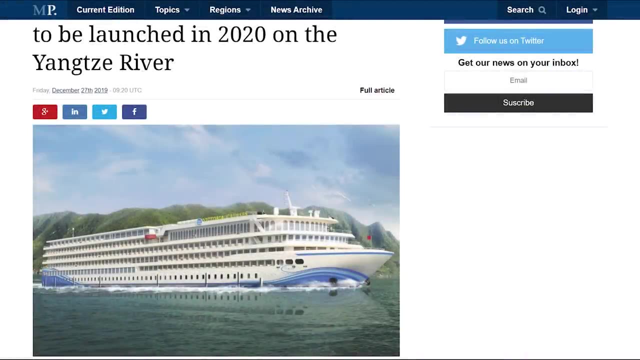 of west africa. during the dry season, even the niger will carry barges weighing no more than eight tons. by contrast, ships weighing ten thousand tons can go hundreds of months to the east and the west to the west and the west to the east to the west and the west to the 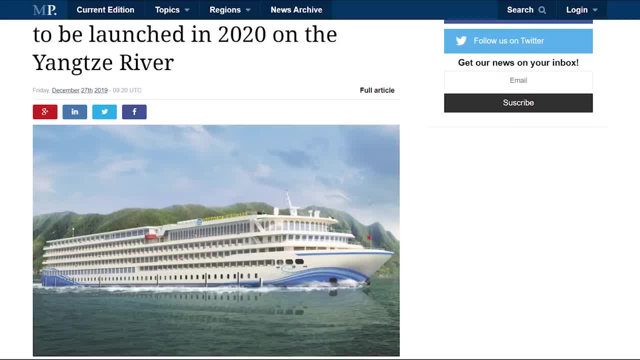 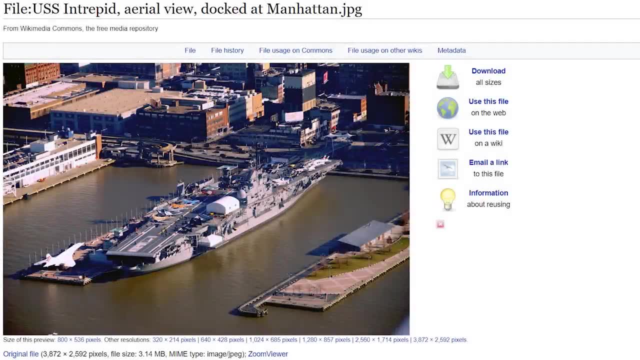 west miles up the yangtze river in china and smaller vessels another thousand miles beyond that. aircraft carriers can go up the hudson river and dock at a pier in mid-manhattan. navigable rivers in africa seldom mean anything approaching that. even the nile was unable to. 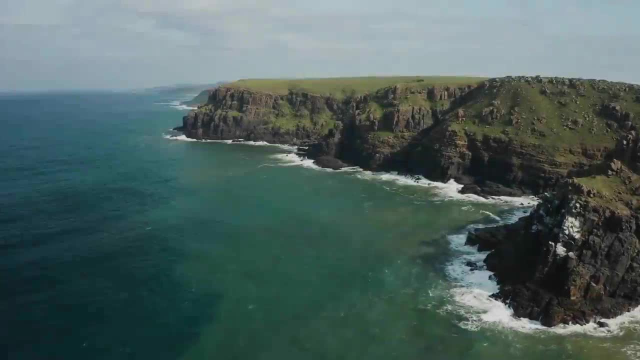 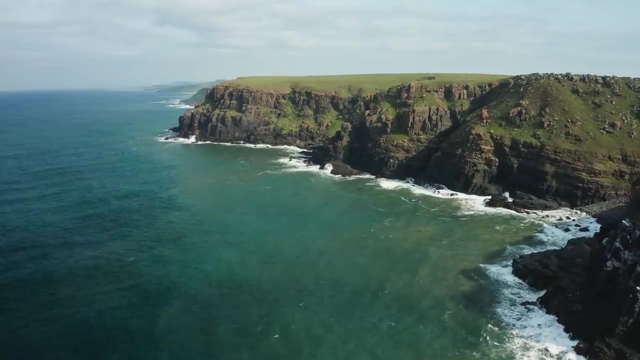 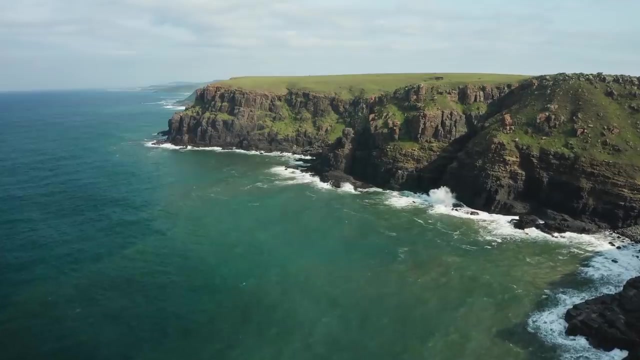 handle the largest vessels in roman times. moreover, because so much of tropical africa consists of high plateaus, almost the entire continent is more than 1 000 feet above sea level and half the continent is more than 2 500 feet above sea level- african rivers must plunge greater vertical. 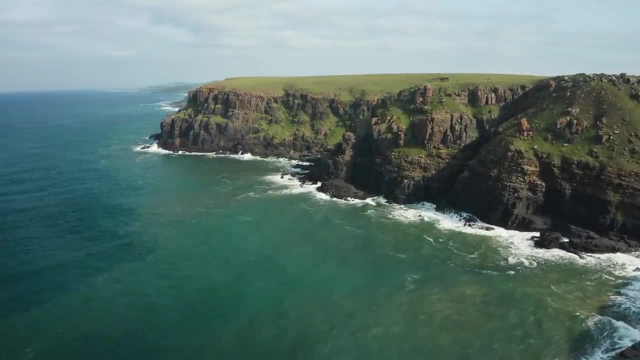 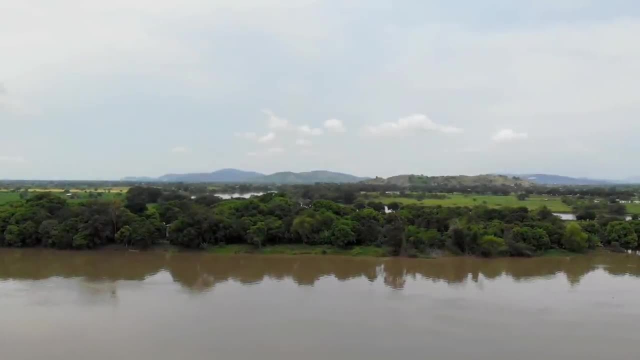 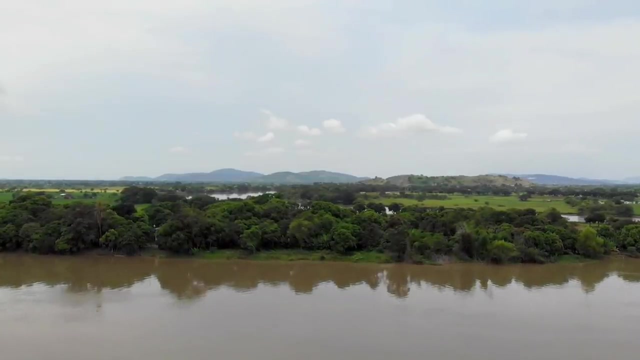 distances to reach the sea, making them less navigable on route. while the amazon river falls only about 20 feet during its last 500 miles to the sea, the zaire river drops about a thousand feet and 250 miles as it approaches the sea. as a geographer has put it, the african 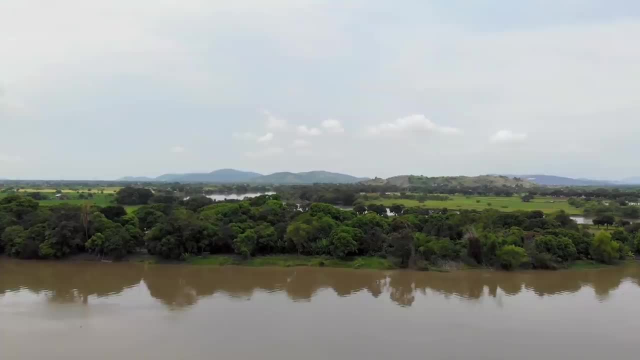 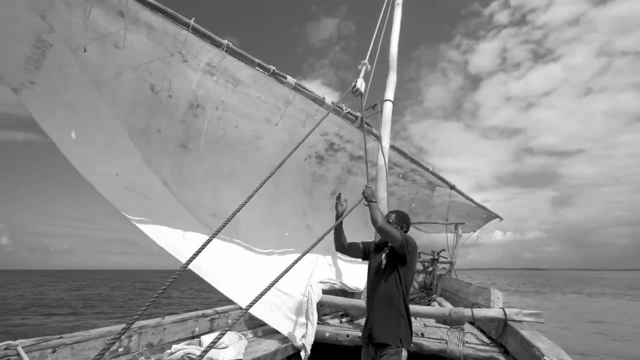 continent is cursed with a mesa form which converts nearly every river into a sea of stars, to become a into a plunging torrent. However impenetrable much of the interior of sub-Saharan Africa may have been to large ocean-going ships, the continent's coastal waters have been plied. 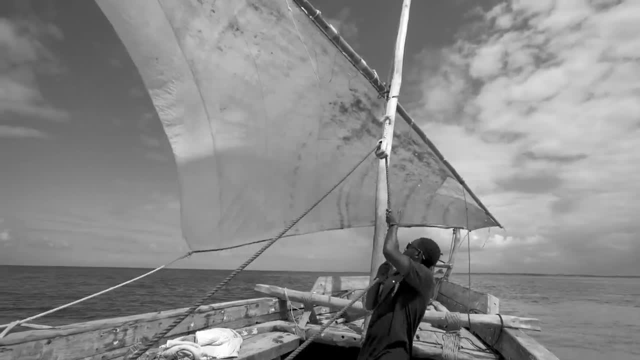 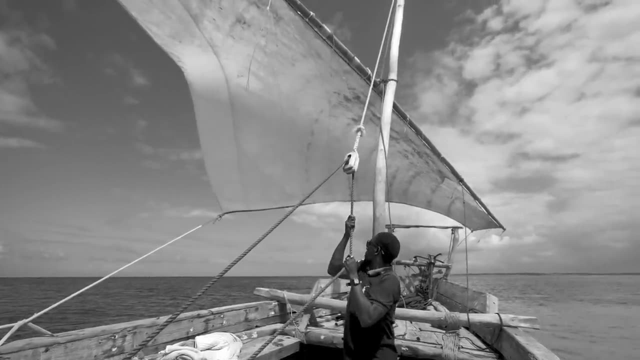 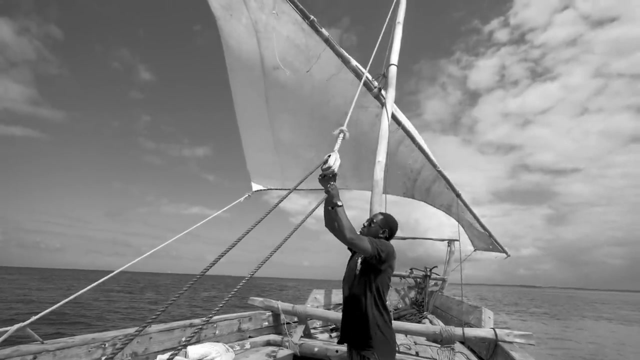 by smaller boats, which could and did go inland as well, being unloaded and carried around waterfalls. Shipments from ocean-going vessels could also be loaded onto smaller craft for transportation into the interior on rivers. Local water-borne traffic between inland locations was likewise possible by carrying boats and their cargoes around rapids and waterfalls. 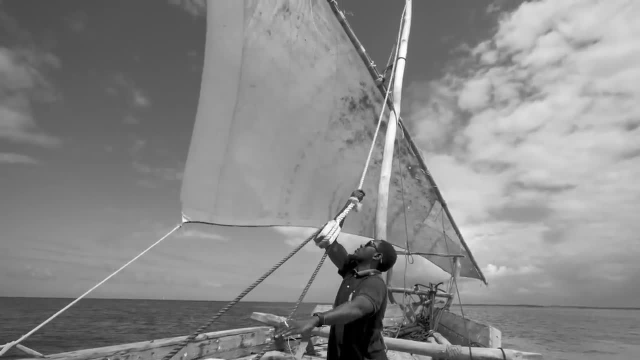 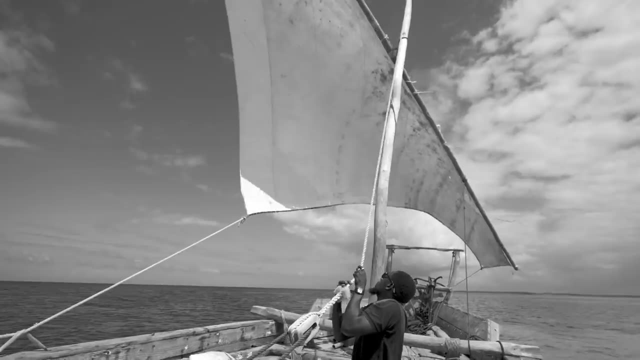 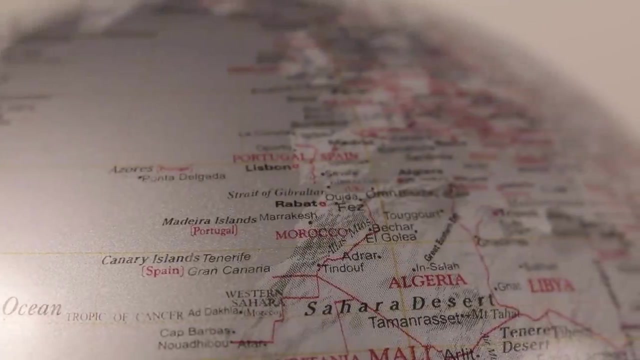 Sometimes these boats and cargoes were carried from one river to another, thereby expanding the reach of commerce. For example, an overland route requiring twenty-five days of porterage on land connected the Niger and the Senegal rivers in centuries past. Moreover, even rivers beset with 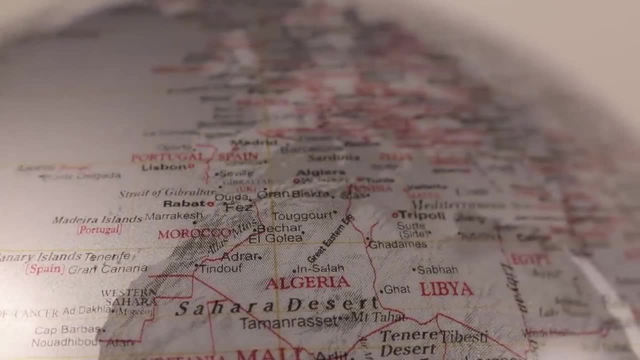 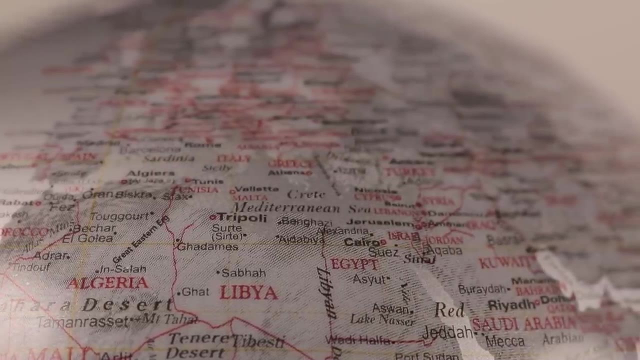 cascades and waterfalls may have navigable stretches that add up to considerable distances: Hundreds of miles on the Senegal and more than fifteen hundred on the Zaire, even though these are not continuous distances. Thus, the various regions of Africa were not hermetically. 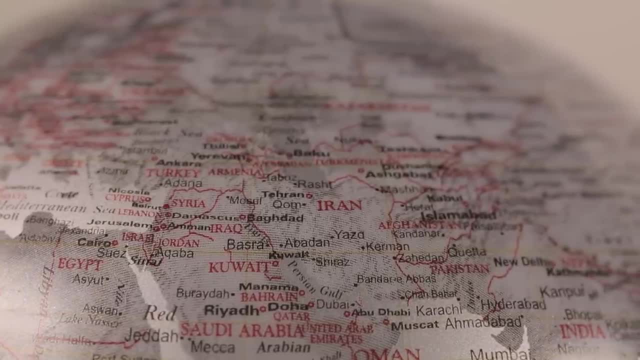 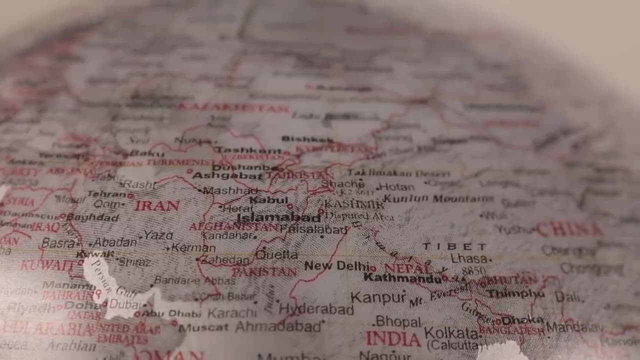 sealed off from one another or from the outside world, but both the volume and the variety of trade, as well as the distances involved, were nevertheless severely curtailed in comparison with more geographically fortunate regions of the world, where heavy and bulky cargoes 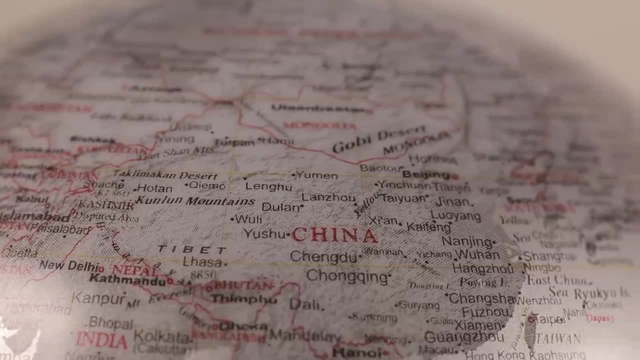 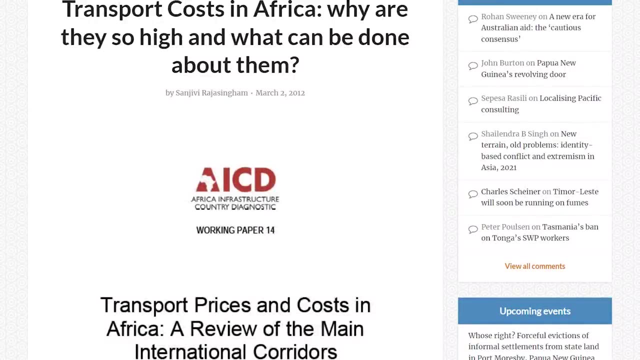 of coal ores and grain were not readily available, and grain could be shipped long distances in continuous river and ocean voyages. A late twentieth-century comparison of the transportation costs of grain in several Asian and African nations found that these transport costs were a higher proportion of the total price. 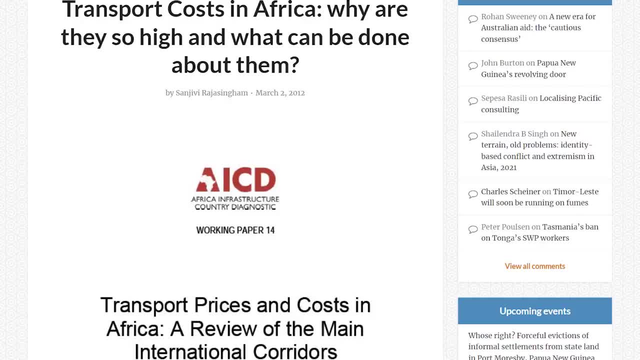 paid for grain by consumers in Africa. Moreover, such statistics do not capture the effect of transport costs on grain that was never shipped in the first place, precisely because higher shipping costs would have made it prohibitively expensive. Contemporary transport costs also cannot capture the handicaps created by even higher transport costs in Africa before many. 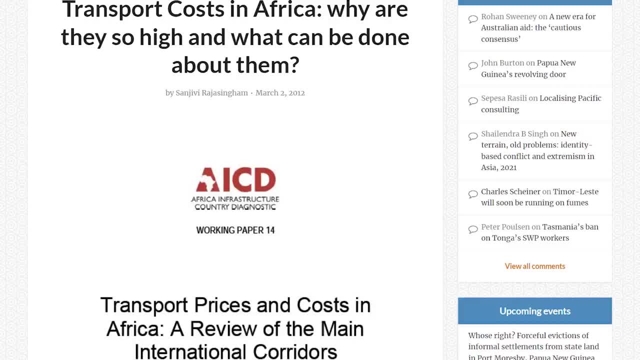 of the transportation advances from the rest of the world were introduced in the nineteenth and early twentieth centuries, and before African harbors could be dredged by modern European equipment and Western railroads built. While it is true, as an historian has said, that 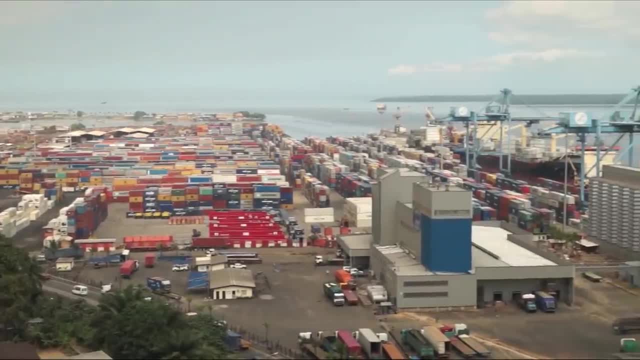 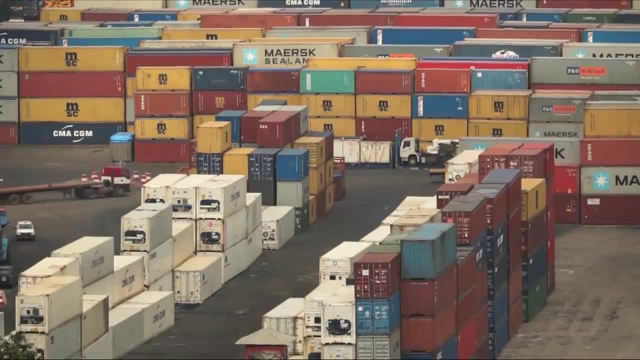 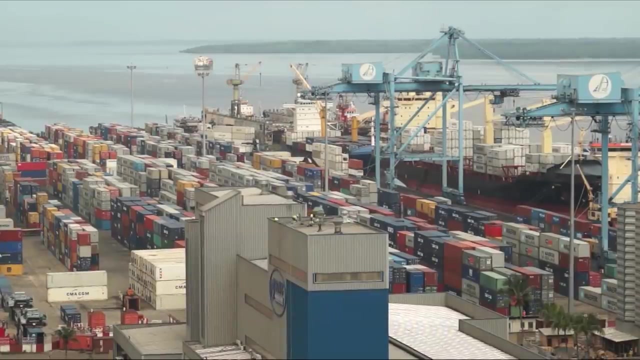 a considerable portion of West Africa was built in the late nineteenth-century. Africa was part of a hydrographic system that was ultimately connected to the Atlantic. the limitations of that system are a part of the story that cannot be omitted without serious distortion. Moreover, the distances between the interior hinterlands and the open seas, 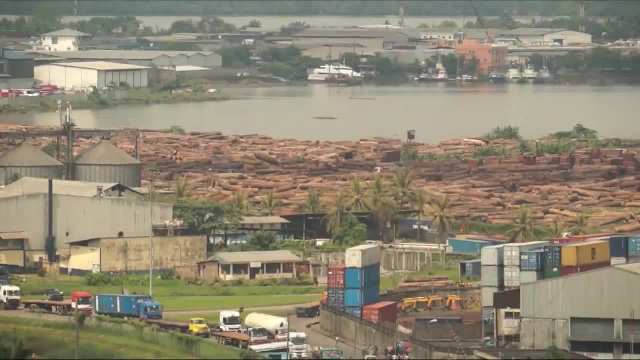 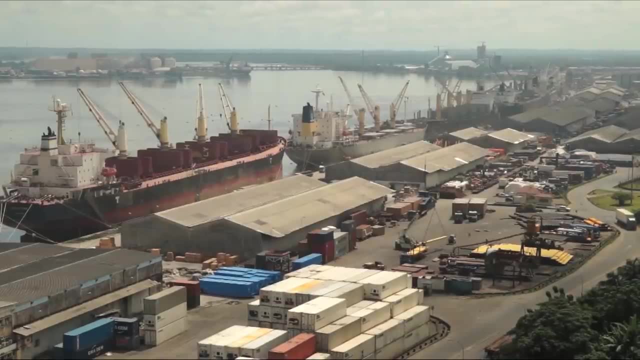 are greater in Africa than in Europe, for example, while the means of covering those distances are much more limited by geography. in Africa, In Europe, no part of the continent outside of Russia is more than five hundred kilometers from the center of the Atlantic. 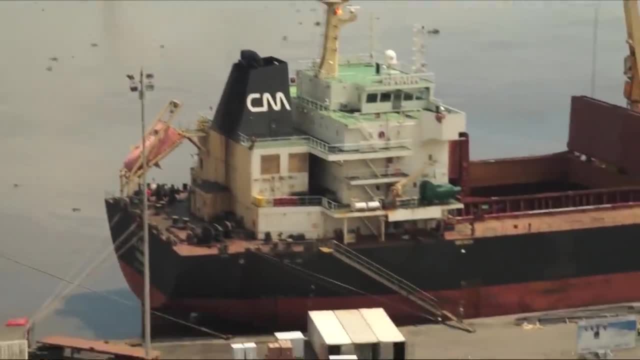 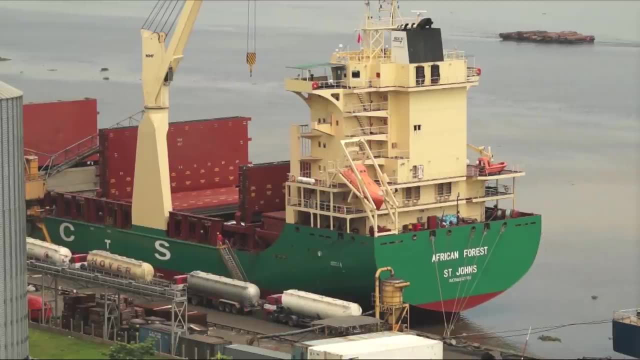 but a substantial part of tropical Africa is more than five hundred miles from the sea and a portion is more than one thousand miles from the sea. Only Asia has a larger interior area remote from the sea, though Asia has more navigable rivers connecting its interior. 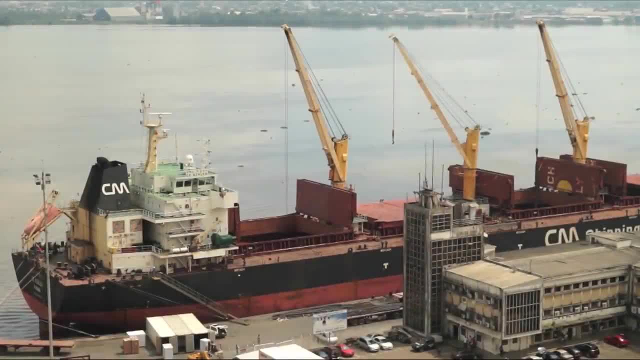 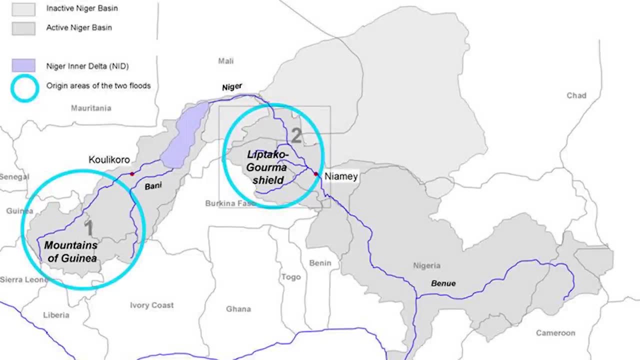 with the coast. The geographical positions of African rivers must also be taken into account. Although the Niger River originates just two hundred miles from the Atlantic Ocean, it circles far inland before it reaches the Atlantic Ocean. This is because the sea is more than one hundred kilometers from the center of the Atlantic Ocean and it covers 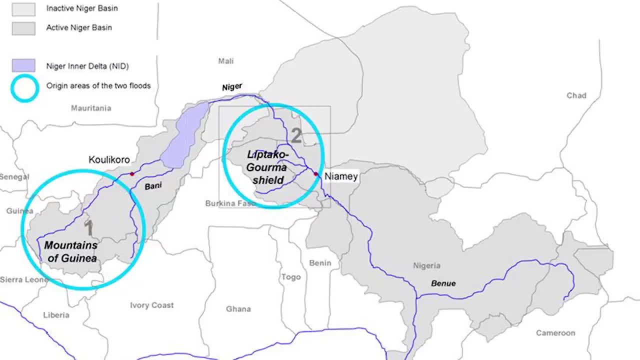 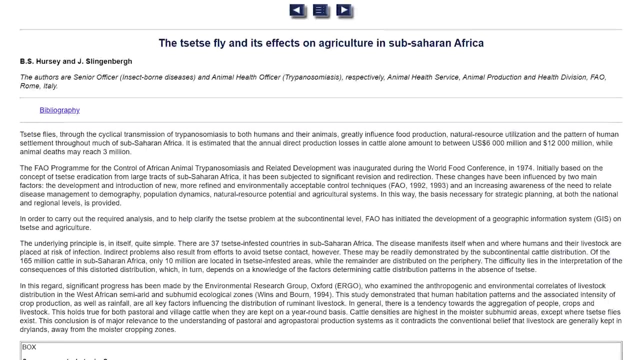 twenty-six hundred miles before actually reaching the ocean. In general, the tenuous connection of the African interior with the sea has been one of the major geographical barriers to the economic, cultural and political development of the continent south of the Sahara. Land transportation in large regions of sub-Saharan Africa has also been made more difficult because 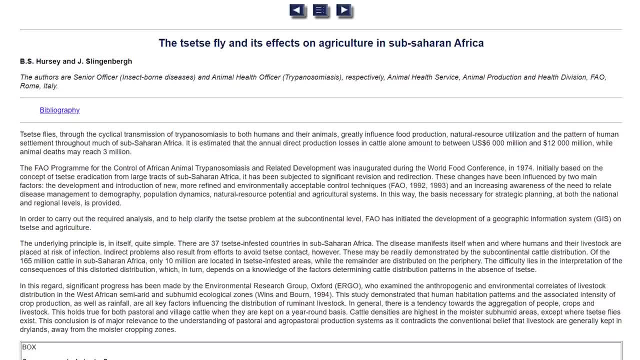 of the prevalence of the tsetse fly, which has carried a far greater number of people away from the discovery of radical and asthma-inducing diseases. As a result, the use of the land transportation system has led Africa to be more vulnerable to food shortages and more. Schutz, as said, as a common common malignant disease. One of the major causes of this is the non-existence of the tsetse fly, which has also led to the spread of the disease across the entire Pacific Ocean. Aliso is also known as the number one Malian bacteria. 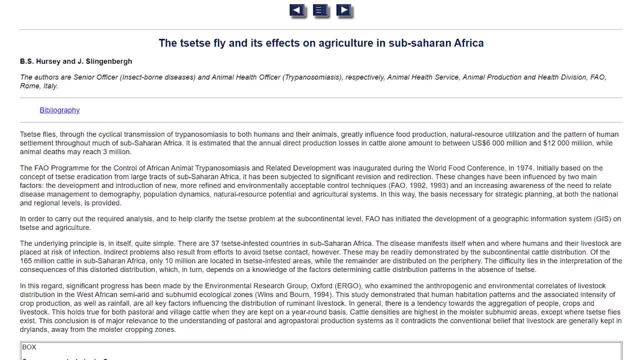 in Africa and is a common strata of African disease. The распarilla will 제품atization of the tsetse fly is a common disease. that is common for some, but is also a common disease in most other species. 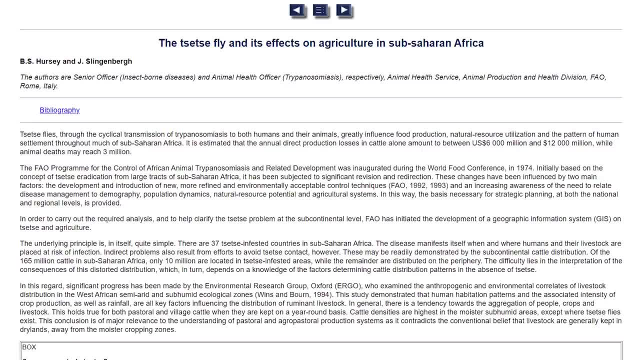 On average. many species oflington people are connected to its form, which is most likely to be due to an abnormal body temperature, With the effect of the buddies of the tsetse fly, the tsetse fly'swirth and its 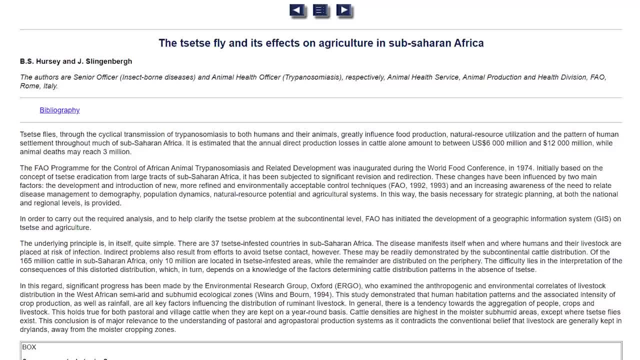 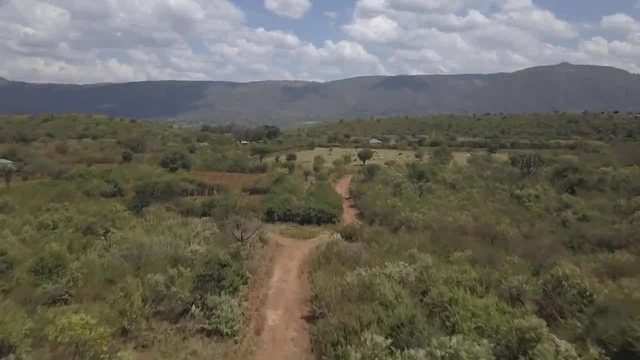 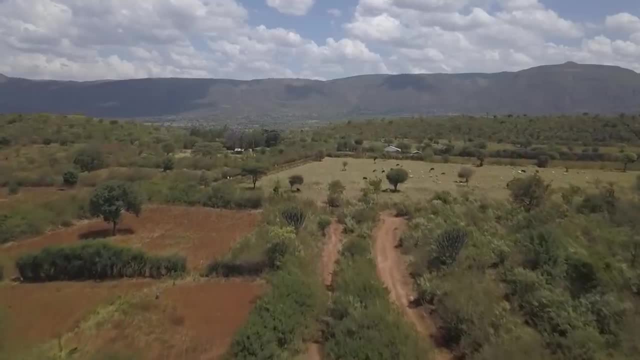 bleak alternatives left to them, without the help of either the waterways or the animal power available. to other peoples on other continents, Expensive transportation provided by human beings limited what could be carried, how far it could be carried and how fast. In addition to the physical limitations, there were narrower limits imposed by economics. 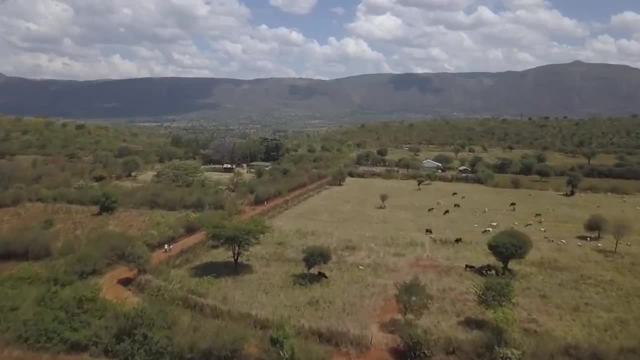 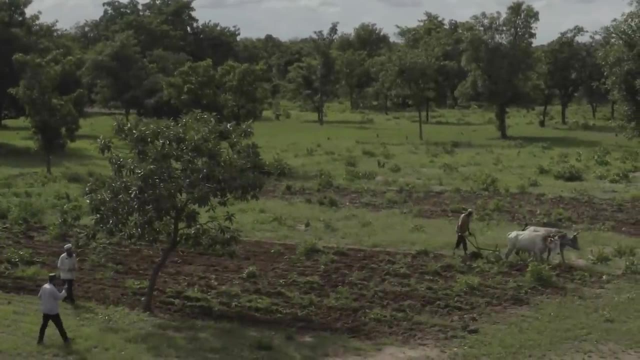 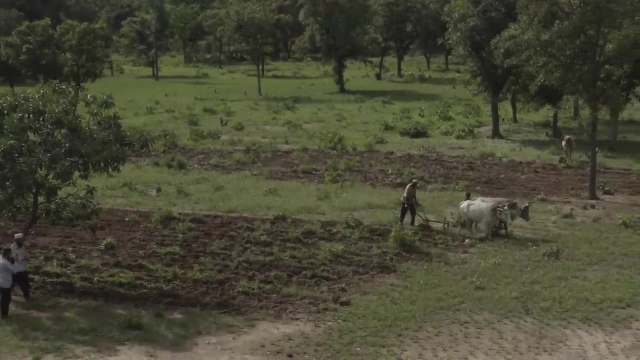 as to what items contained enough value in a relatively small space to repay the costs of this expensive method of transport. The lack of animals' muscle power in tropical Africa has been felt not only in transportation, but also in farming. A dearth of draft animals in farming often meant not only a loss of 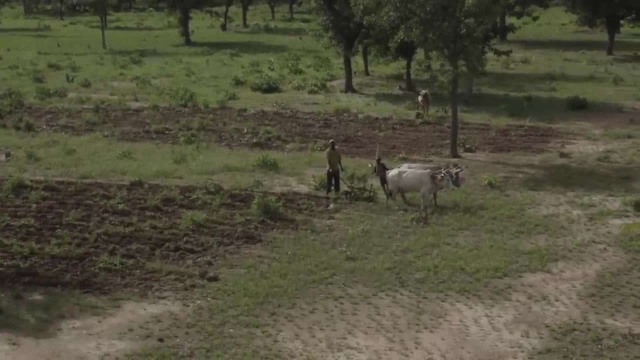 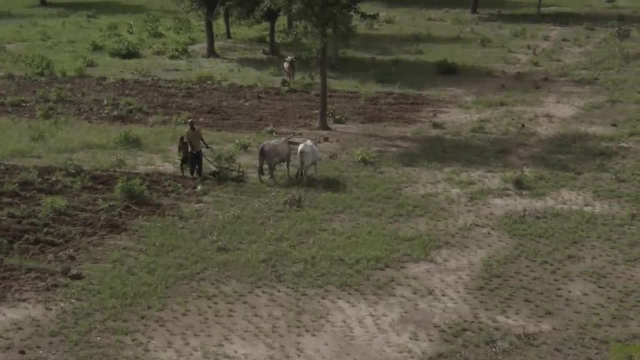 muscle power, but also a dearth of fertilizer. The latter has been especially important in those parts of the continent where soils have been very much in need of fertilizer, because their low nutrient content and proneness to erosion meant that their fertility was at a very high risk of deterioration. 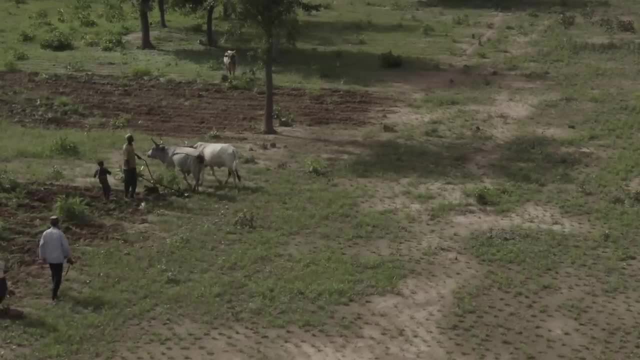 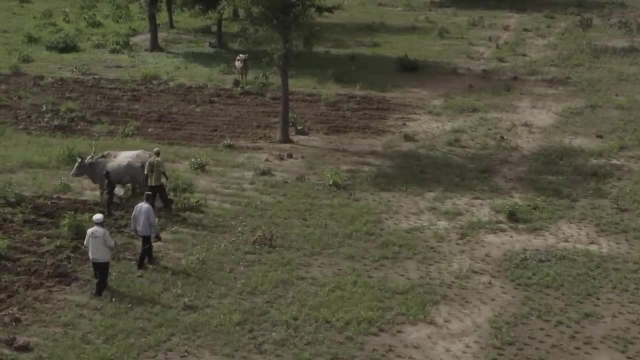 The soil was also very dry and its fertility was easily exhausted by cultivation. Rainfall patterns in parts of Africa—long dry spells followed by torrential downpours—increase erosion, since dry baked soil is more easily washed away. Moreover, these torrential tropical 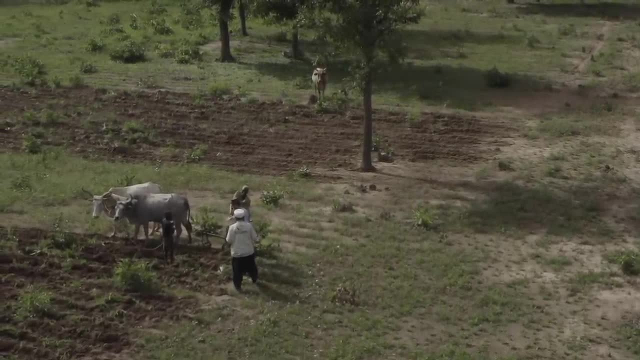 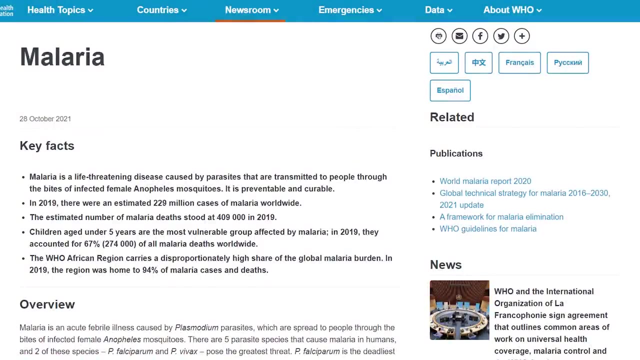 downpours tend to leach the nutrients from the soil, in Africa as in many other tropical regions. Finally, the tropics provide a disease environment in which many more deadly diseases may flourish or expand into some other areas of the continent, Since the geehrt of tropical climates have caused theți of seas to Consumption. when 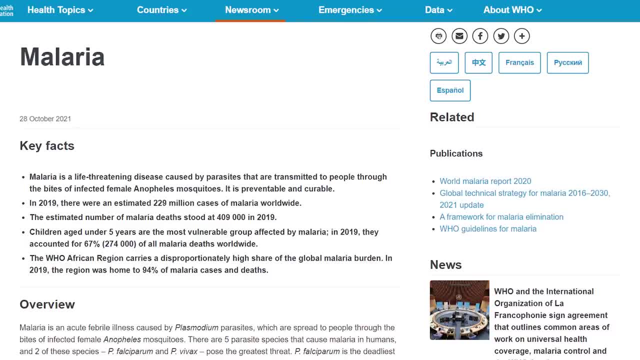 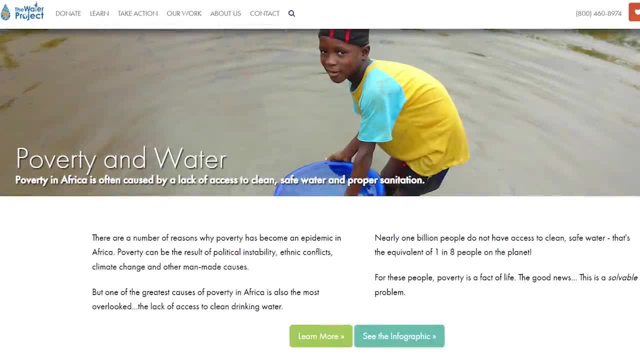 there is pushed down from the water, or il Bi, somehow led to death. for example, 90 percent of all deaths from malaria in the world occur in sub-Saharan Africa. Even a listing of individual geographical disadvantages in Africa may understate the handicaps they represent in combination. For example, the problem of poor water transportation—while 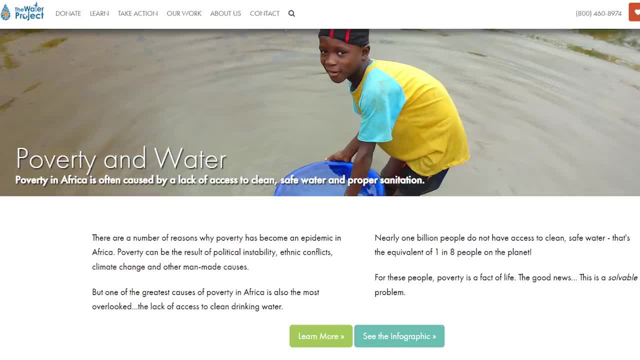 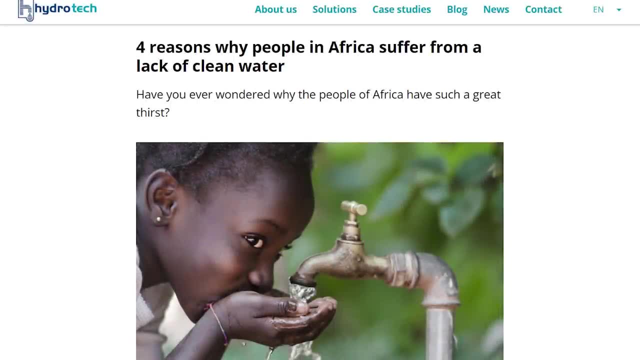 serious in itself—is still more serious in combination with poor land transportation across much difficult terrain without the aid of pack animals. The highly variable rainfall patterns become more serious in view of where the rain falls. A geographical study of Africa found plenty of water available where it cannot be used and a scarcity where it is most needed. 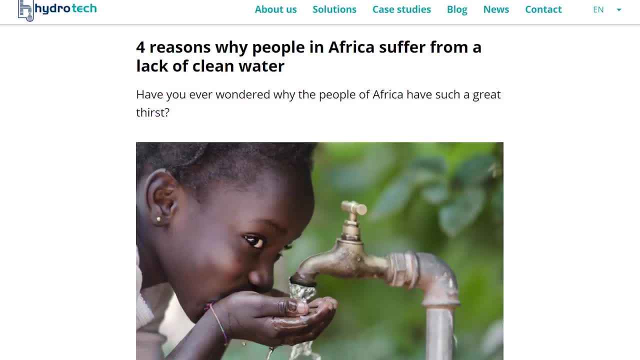 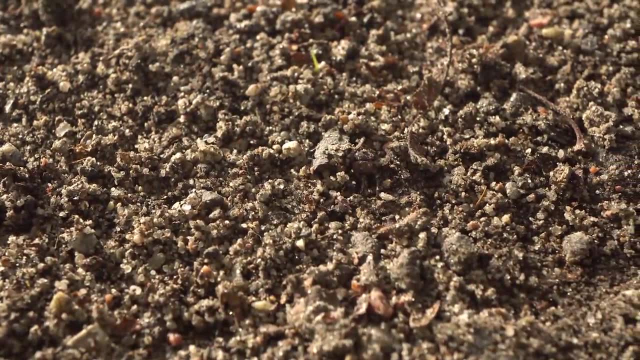 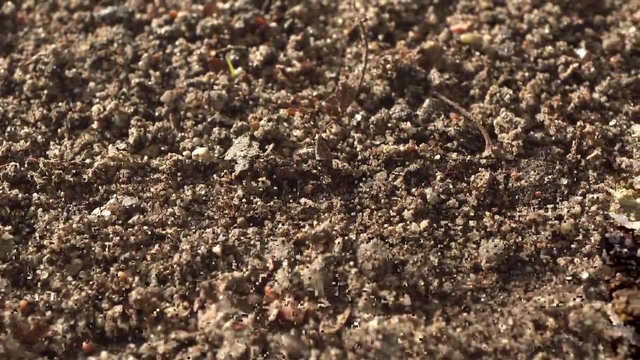 Not all parts of sub-Saharan Africa have suffered all these disabilities simultaneously. However, the fragile fertility in some regions of tropical Africa has meant that a given territory would not permanently feed people at a given location, and this in turn meant that those people had to move on every few years to find new land that would feed them while the land they 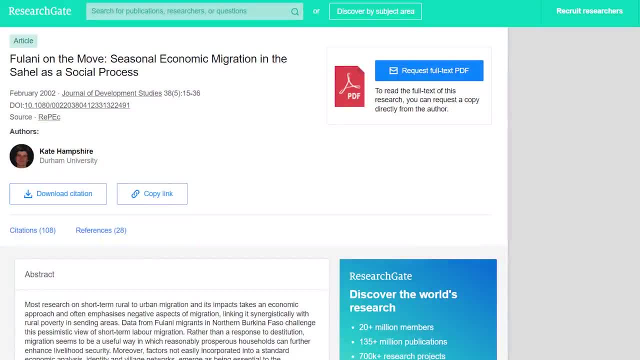 left behind recovered its fertility. Therefore, whole societies had to be mobile, foregoing the opportunities to build territorially based communities with permanent structures, such as other Africans built in more geographically favored parts of the continent and which were common in Europe, Asia and Africa. 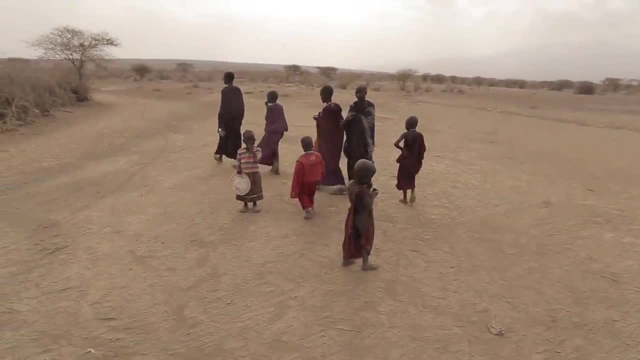 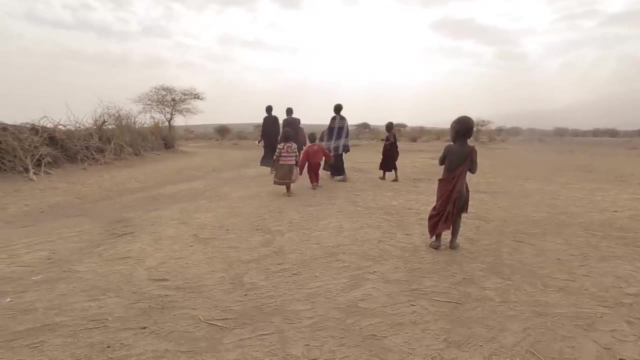 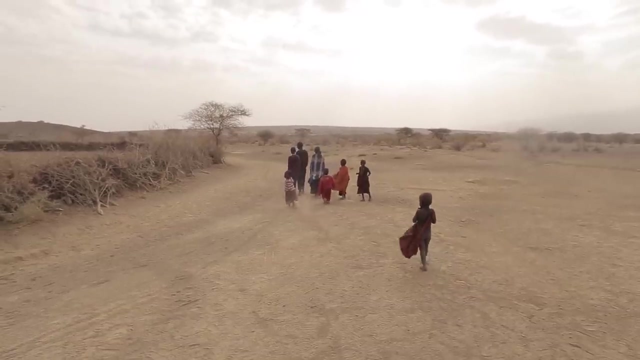 The provincialism of isolated peoples has not been peculiar to Africa. What has been peculiar to Africa are the geographic barriers to mobility that have pervaded vast areas below the Sahara. Waterways extend the boundaries of cultural interchange, but in much of sub-Saharan Africa 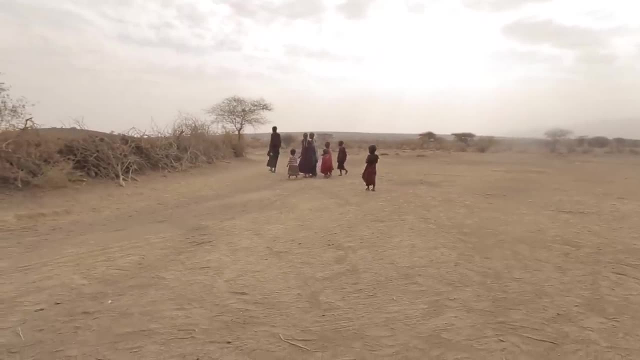 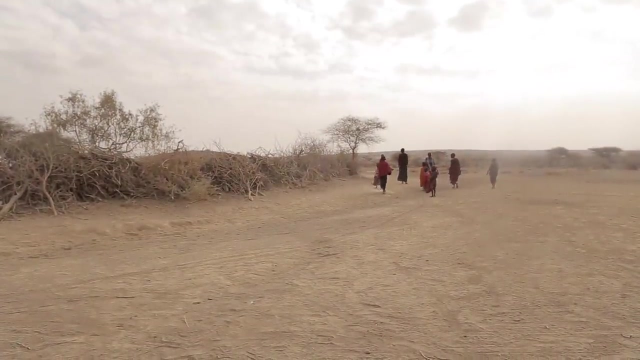 they did not extend those cultural boundaries very far, Like other places relatively isolated from broader cultural developments- the Scottish Highlands, the Scottish Highlands, the Scottish Islands, parts of the Balkans or the South Sea Islands, for example, much of sub-Saharan Africa. 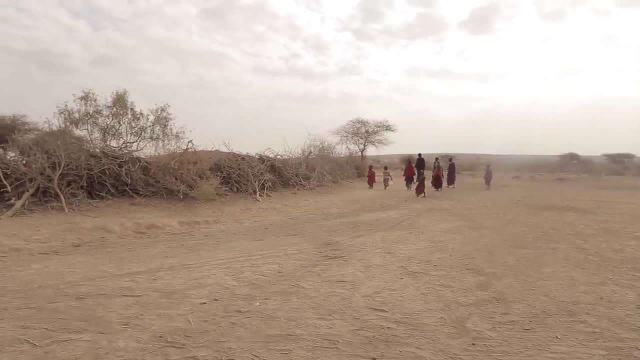 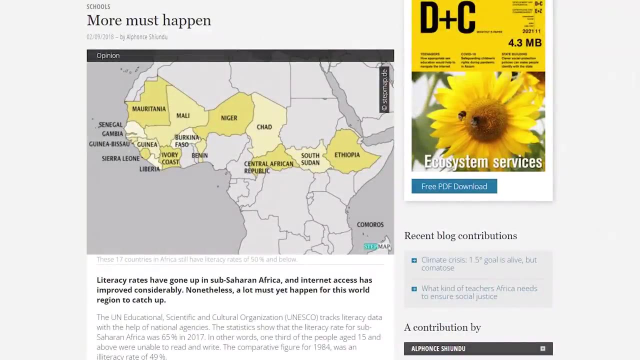 tended to lag behind the technological, organizational and economic progress in other parts of the world. A lack of literacy throughout most of sub-Saharan Africa further limited both internal development and the stimulus of contacts with distant times and places via the written word, While similar retardation afflicted particular parts of Europe or Asia, or isolated. 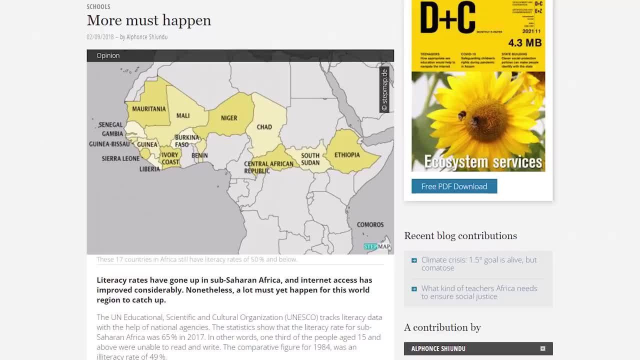 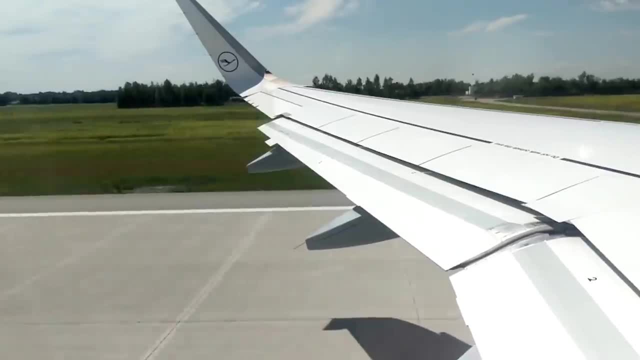 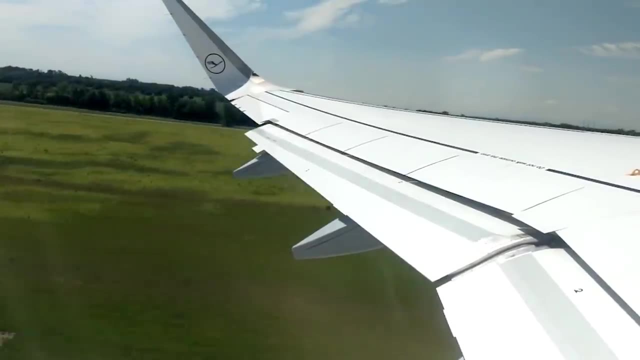 island communities around the world. in Africa, such cultural isolation characterized wide areas and many peoples. The degree of these cultural handicaps has varied in different parts of the continent and has changed over time. Railroads, motor transport and airplanes have all added to. 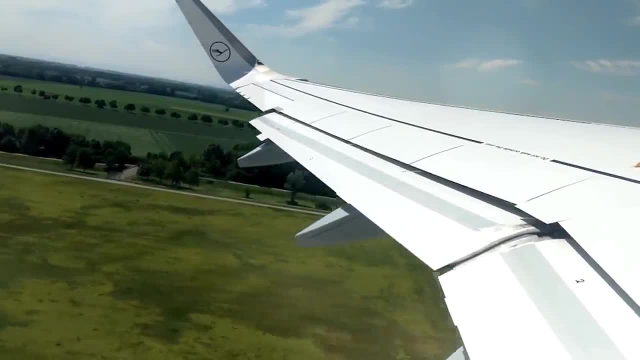 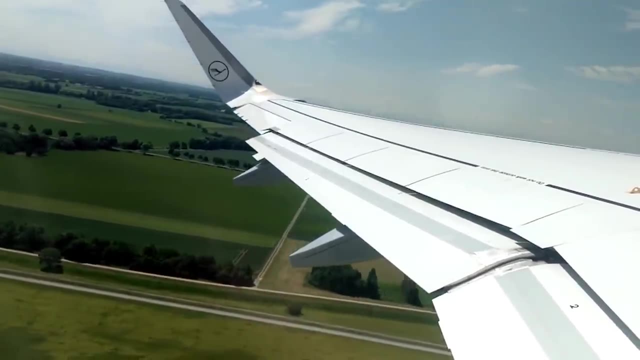 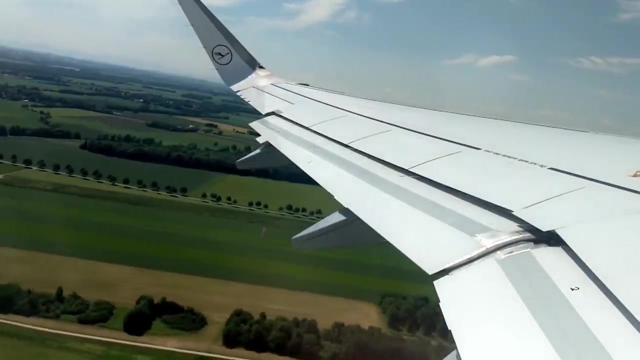 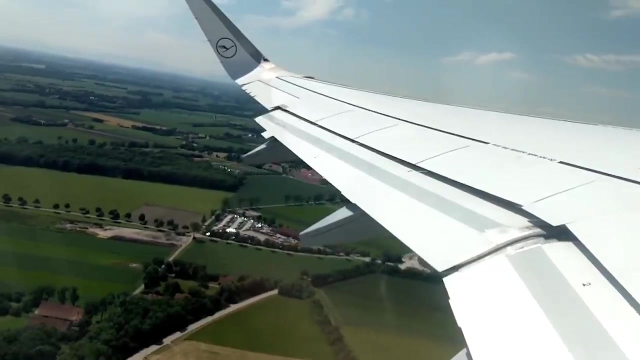 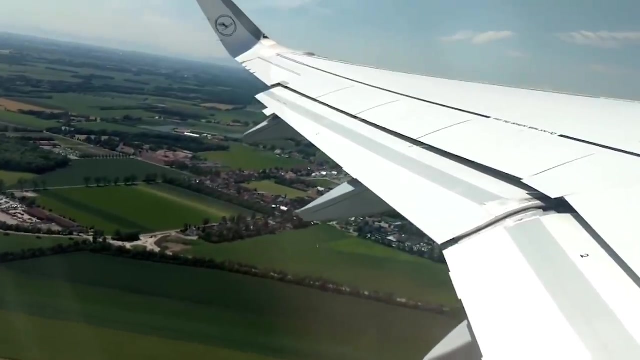 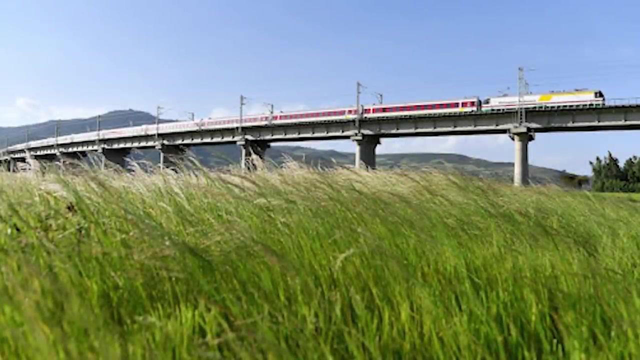 transportation possibilities and electronic communication media, from cheap radios to television, have penetrated cultural isolation, But all this has happened because of the lack of access to the public sector. The rail line from Djibouti to Addis Ababa, for example, rises more than 2,000 feet in its 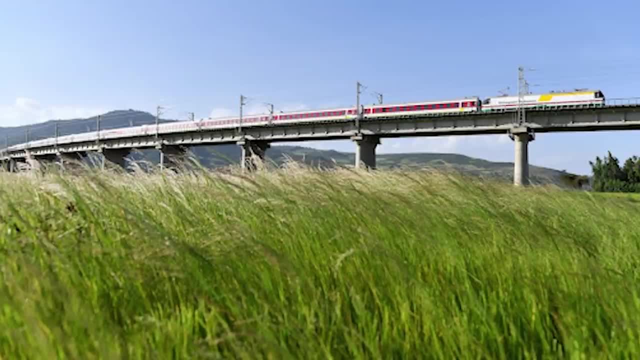 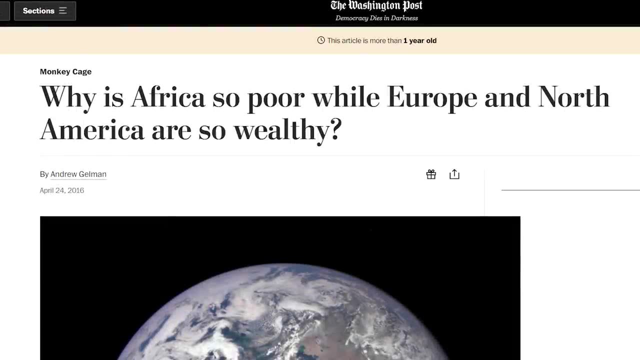 first 60 miles and more than 4,600 feet in its last 180 miles. Given the multiple and formidable geographical obstacles to its economic and cultural development, Africa's poverty is hardly surprising. This poverty over much of sub-Saharan Africa is 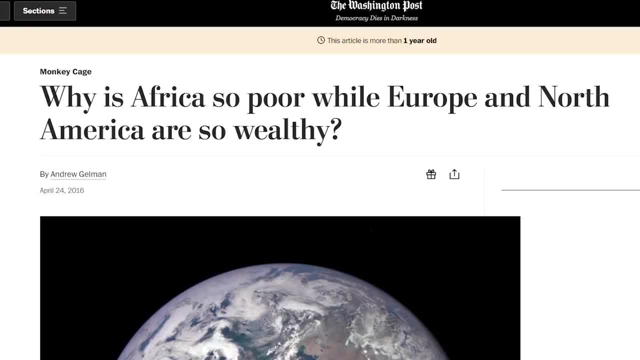 shown in many ways. Lower incomes per capita are an obvious indicator, though the complexities of international exchange rates make these statistics questionable as measures of relative change. However, when the monetary value of output per capita in Nigeria is less than 2% of that in the 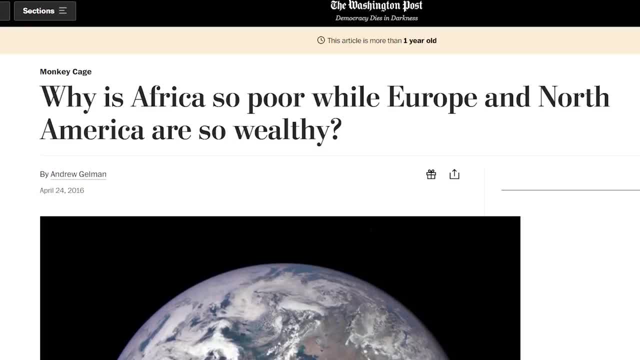 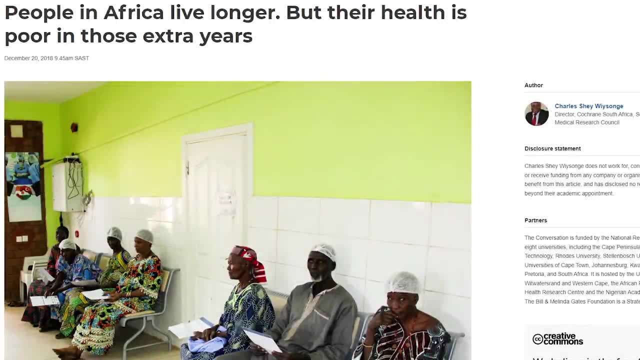 United States and in Tanzania less than 1%. that clearly cannot all be due to exchange rates. A more meaningful picture of differences in living standards is that average life expectancies are typically more than 70 years in Europe, Australia, the United States, Canada and Japan, while average life expectancies in sub-Saharan Africa take about. 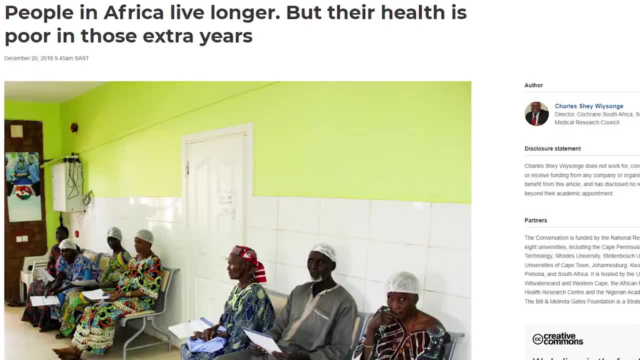 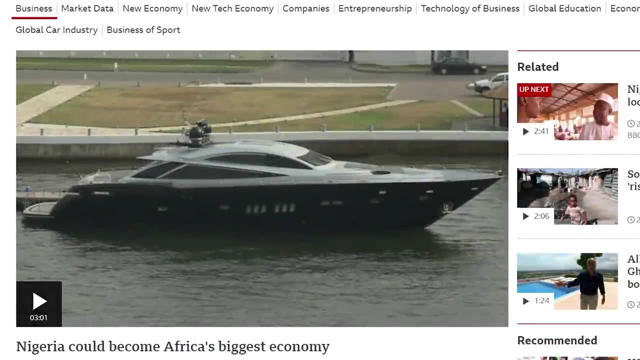 tend to be in the 50s or even the 40s. Moreover, even these life expectancies in Africa have been achieved only with the help of medical and public health measures originating elsewhere in the world. Within this general picture of lagging economic development in much of Africa, there, 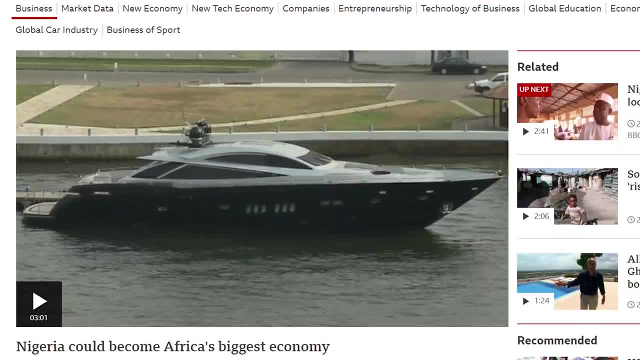 have been historic and continuing variations in economic development and political organization among the various regions of the continent. One of the more fortunate regions of sub-Saharan Africa from various perspectives has been equatorial West Africa, what is today Nigeria, Ghana and their neighboring states. This region has some of the continent's more fertile soil. 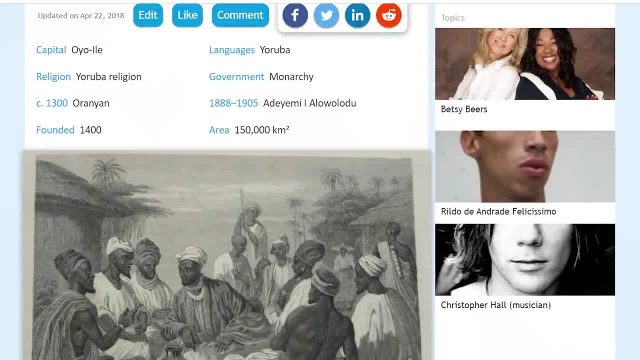 ample rainfall and the Niger River system. Here some of the larger African kingdoms arose. However, even in this relatively more favored region of Africa, the states and even empires that arose were often small by world standards. The Oyo Empire in what is today. Nigeria has been a region of more fertile soil, ample rainfall and the Niger River system. However, even in this relatively more favored region of Africa, the states and even empires that arose were often small by world standards. The Oyo Empire in what is today Nigeria has been 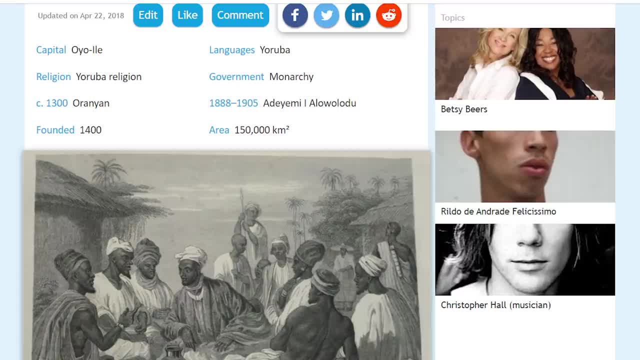 a region of more fertile soil, ample rainfall and the Niger River system. Here some of the major cities of Africa, including Nigeria, covered an estimated 150,000 square kilometers, which is smaller than the American state of Colorado, The Songhai Empire, which included 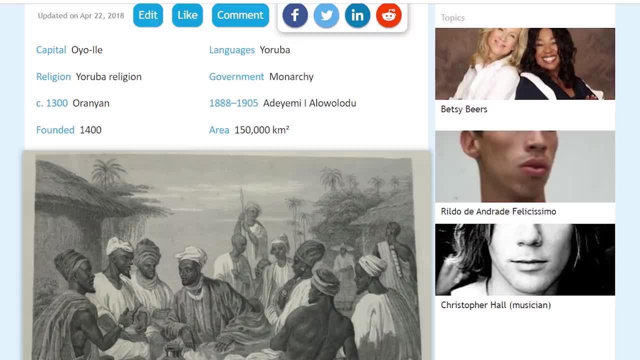 the rich river valleys of the central and western Sudan was about the size of France, which is to say smaller than Texas. Yet these were huge states by African standards, since most Africans lived in polities, only a fraction as large with national populations. 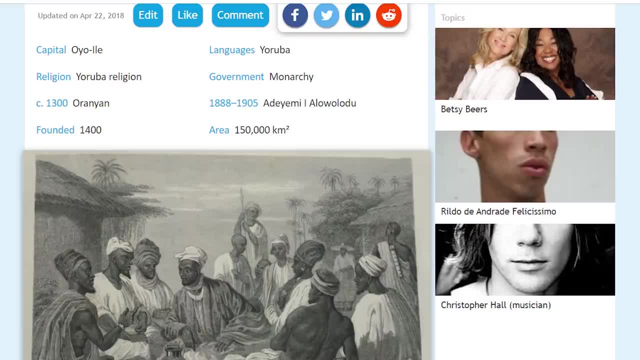 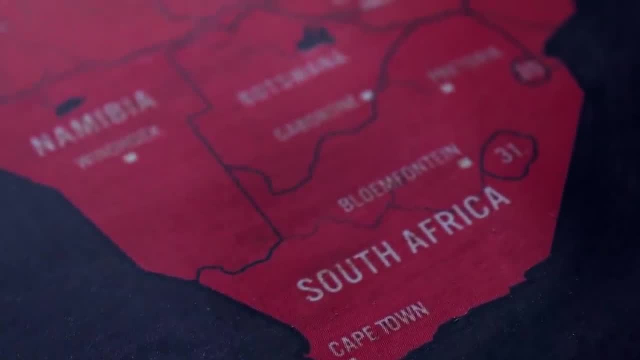 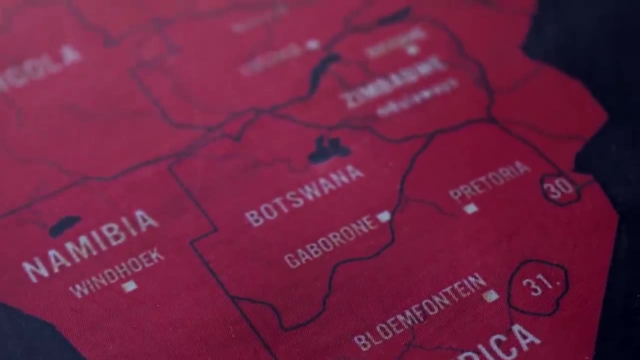 no larger than the populations of cities or even towns in the region. In Africa, as in other parts of the world, those peoples who were more fortunate often used their advantages to subjugate others. In West Africa, this subjugation took the 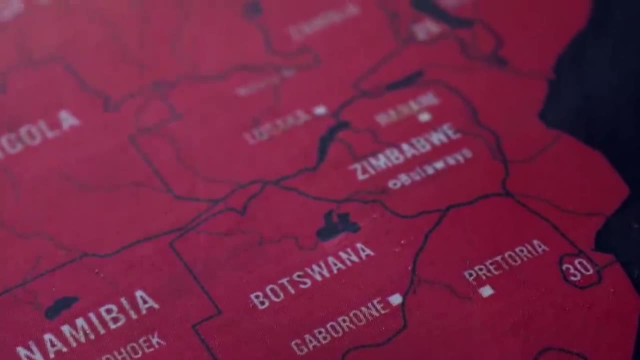 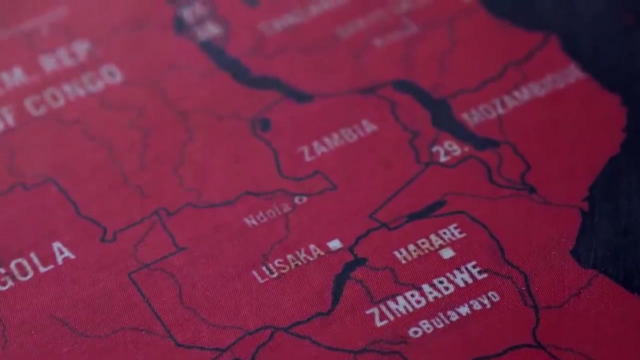 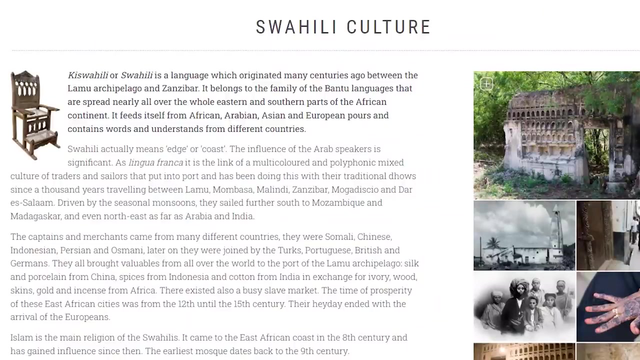 form both of conquest and of enslavement of fellow Africans Across the Sahara in North Africa. more favorable geographic conditions, including harbors on the Mediterranean, also led to larger and more advanced societies. These too were more favorable conditions to subjugate and enslave sub-Saharan Africans In East Africa, some of the more geographically 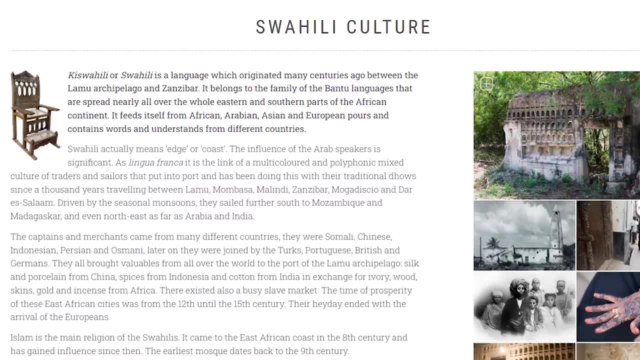 favored areas included harbors such as the large natural harbor on the offshore island of Zanzibar, and such mainland ports as Mombasa and Kilwa. All three became major centers for the trading and shipment of slaves, usually captured from less fortunate inland tribes. 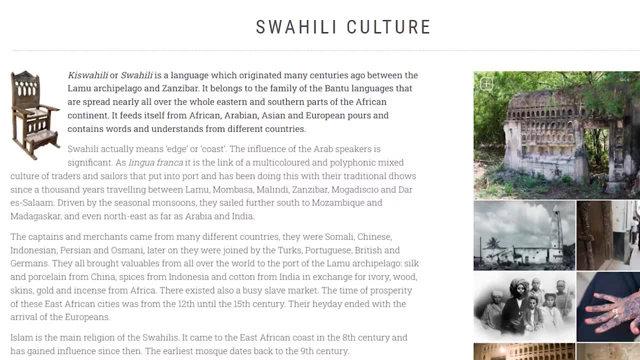 Here, the enslavers were typically either Arabs or people of mixed Arab and African ancestry and culture, known as Swahilis.